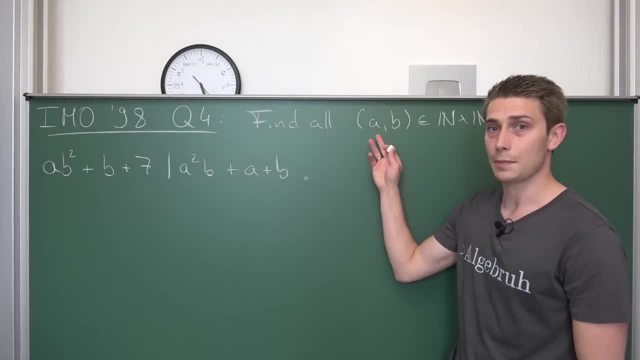 dive right in Now. we are going to find all the ordered pairs, a- b, where a and b are out of the positive integers 1,, 2,, 3,, 4,, 5,, 6,, 7,, blah, blah, blah up until infinity. 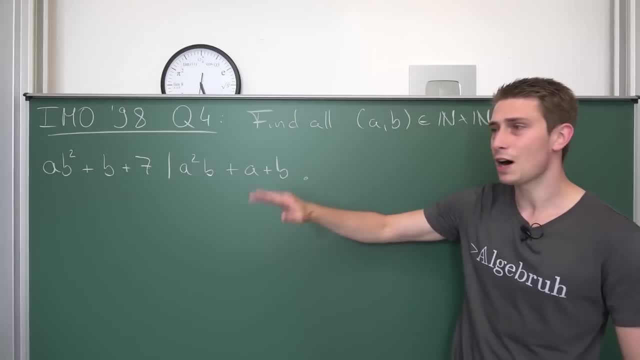 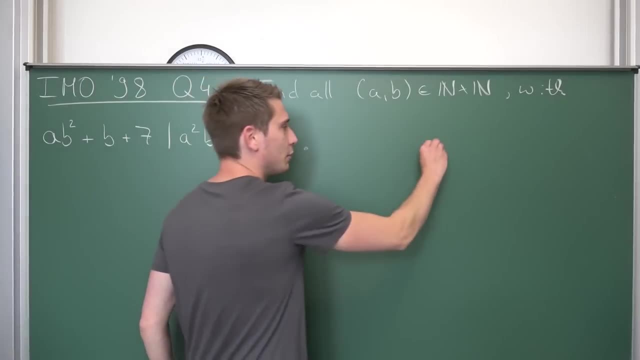 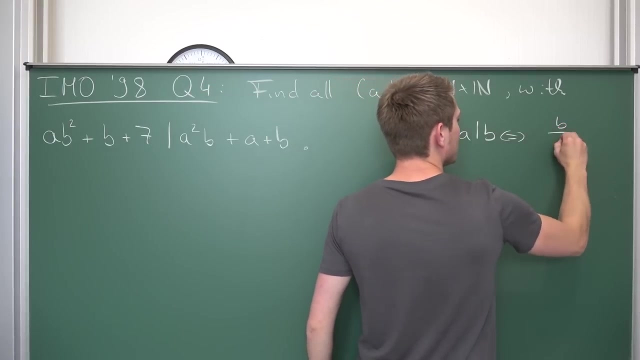 whatsoever, such that a, b squared plus b plus 7 divides a squared times b plus a plus b. Let us at first talk about what divides means. So if we have a divides b, this just means so that's equivalent to saying that we have b divided by a is. 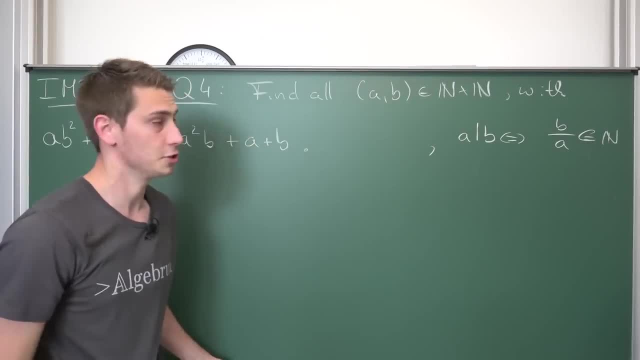 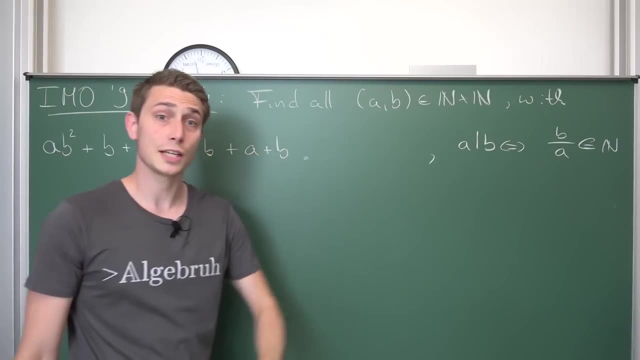 element of integral, In our case the positive integers that we are having here. Okay, a cannot be equal to 0, but this is already stated by our initial conditions. Also, there's one more thing that I would like to take a look at, Namely if we have, for example, 2. 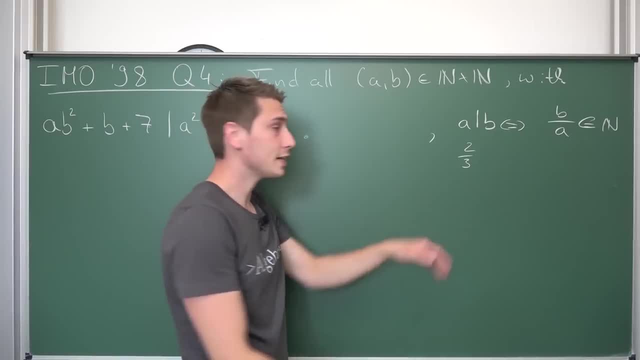 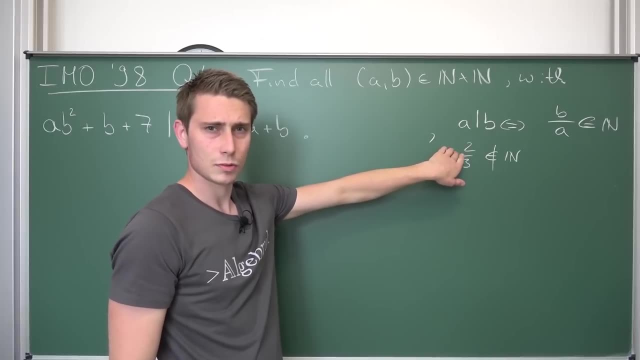 over 3.. Okay, I'm going to give you a few examples here. Then this thing is not element of n, Not element of n, Meaning if our numerator is less than our denominator, we can have an element of n. We have something between 0 and 1 for 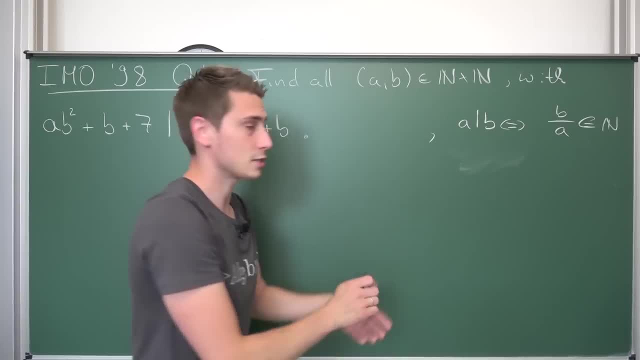 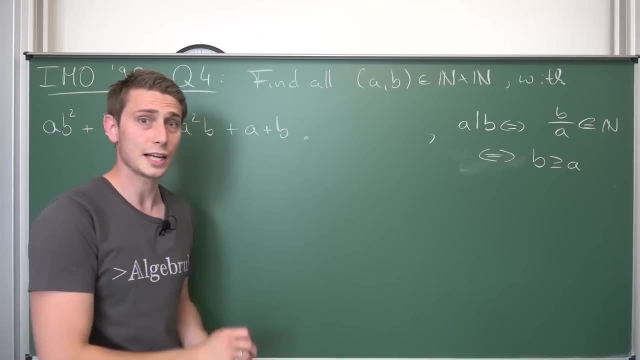 this. So what we can do is we can, for example, say that we have an element 0 and 1 for this, And this is also equivalent to saying that b is greater or equal to a. Okay, Just as a little side note. we are going to need this later Now. 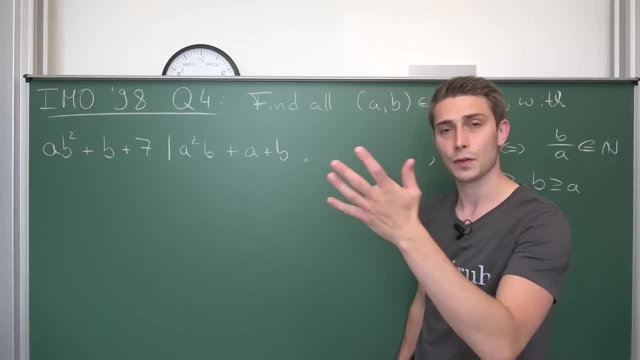 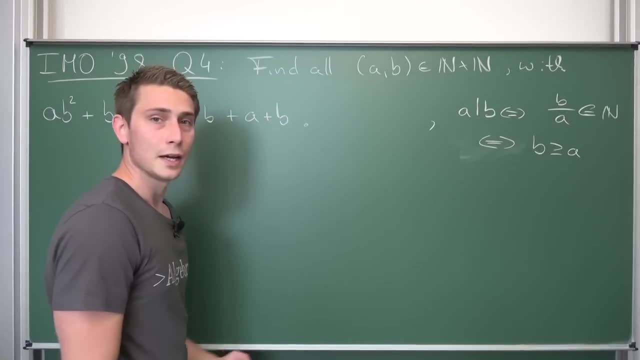 we are going to take a look at what this expression actually means, And here I'm going to use yet again some numbers to make my point more clear. what we are going to do next, what I did next, Or at first I should say So. if we have, for example, 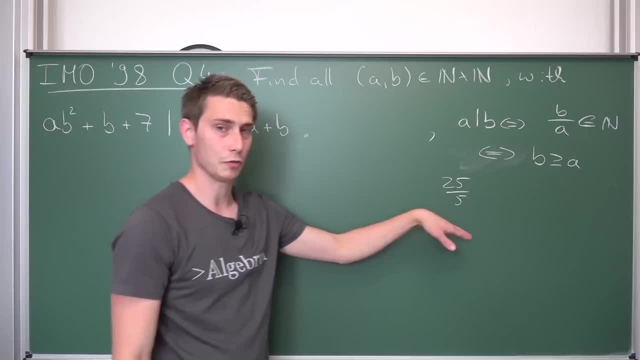 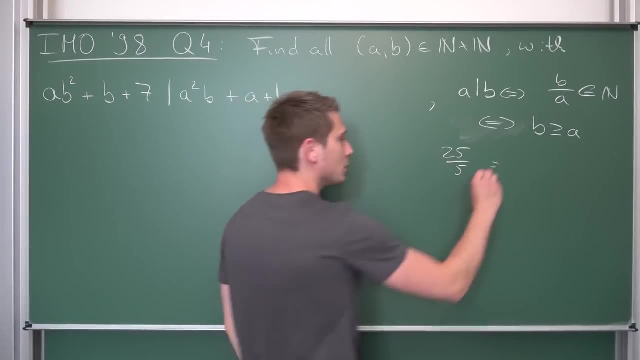 with me that this is element of n, because we are going to get 5 out of it, Meaning in this notation, 5 divides 25.. Now what were to happen if we decompose 25 into, let's say, 23 plus 2, and then over 5.? You might agree with me that if we 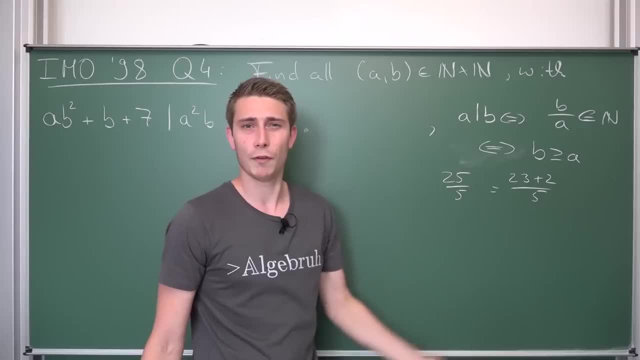 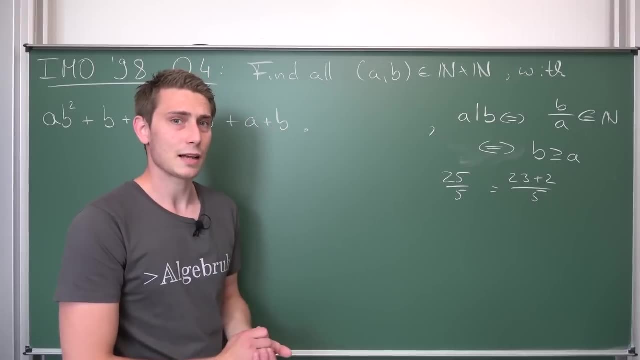 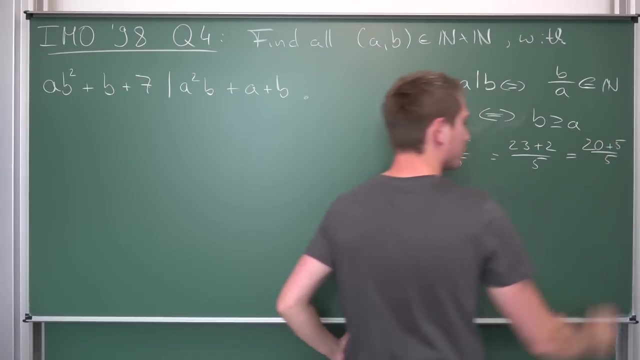 were to use the additivity of our numerator, then 23 over 5 is not divisible- we are going to get a remainder. and also 2 over 5 is not divisible in n. This is not something that does work out, but what happens if we have so 20 plus 5 over 5, that this means that 20 over 5 is going to give us? 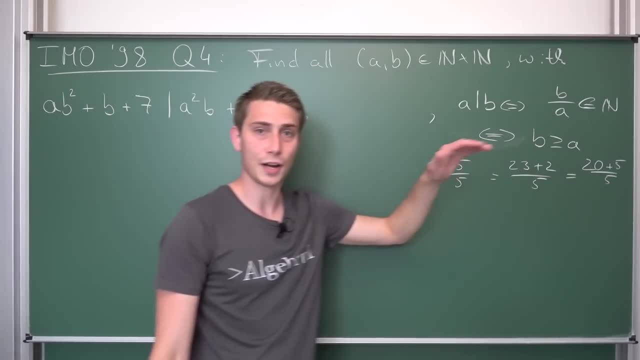 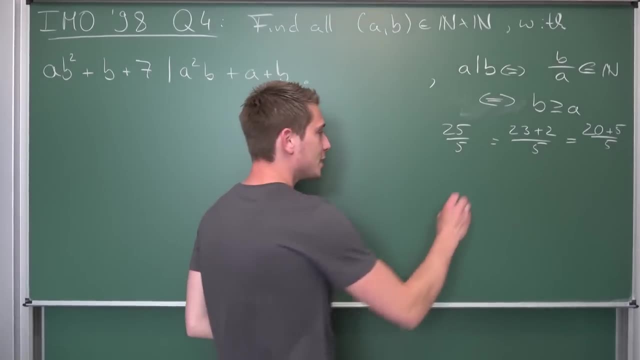 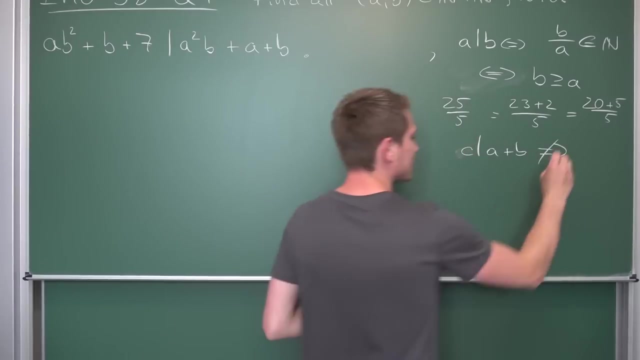 4, it's divisible. and we also have that 5 over 5 is 5 over 5 is 1, which is also divisible. yet again in n. What I want to get at is that in general it doesn't hold that if, let's say, C divides a plus b, this does not imply immediately that 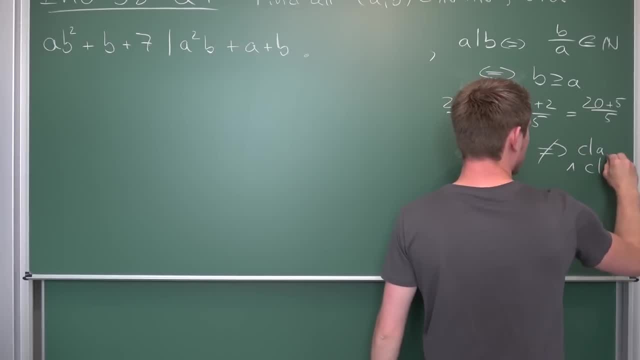 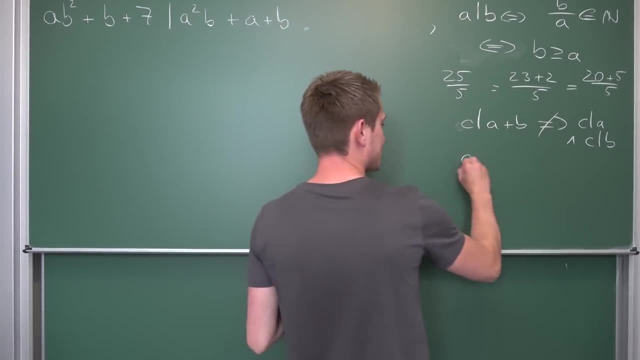 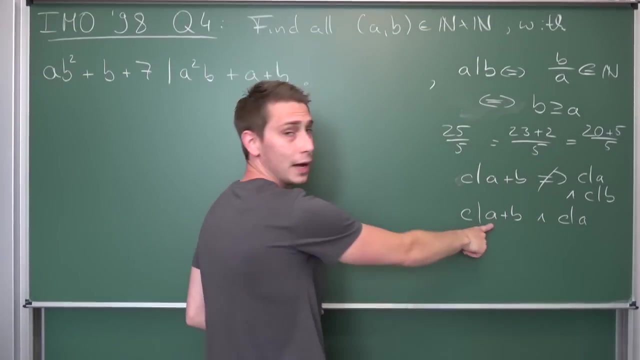 C divides a and we have C divides B. So let's work on this. But if we have a certain decomposition like this one right here, stating, for example, that C Divides a plus B and we have C divides a- this is our case here- So a, in our case, is 20 and our C would divide 20- then this would immediately imply: 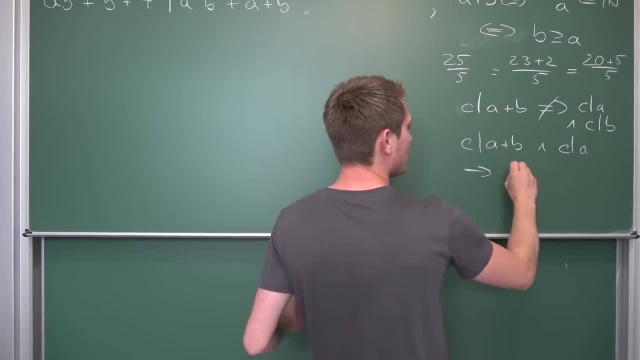 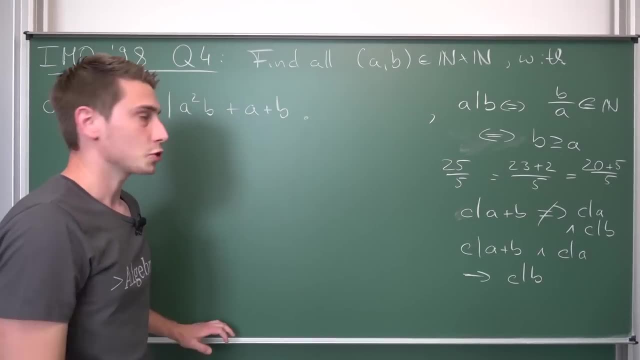 Okay, this is why I'm giving you numbers, because it's easier to understand that we have: C divides B in our case, So 5 divides 5, and this is what we are going to use here. We are going to decompose what we have here. 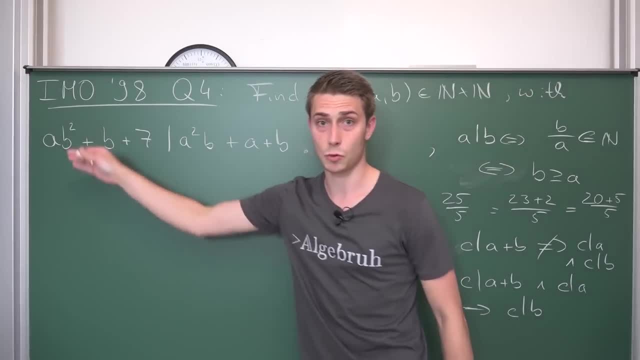 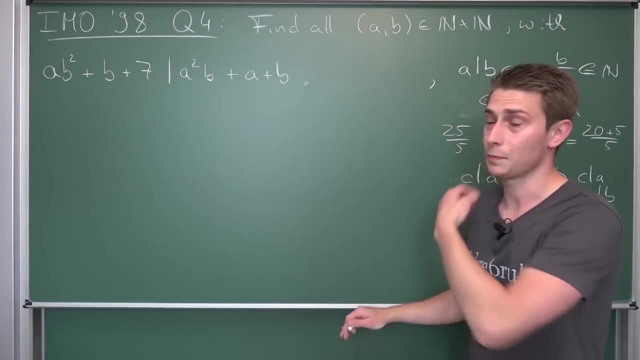 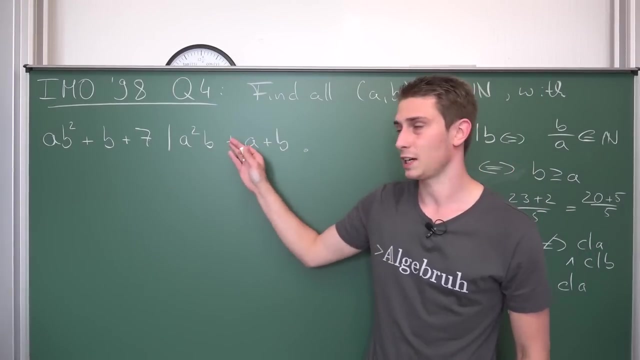 Okay, as our numerator, into something that looks like this right here, and then we can use the additivity, This additive property that we have here, to actually reduce the problem to something easier. This is how I approach it in the first place. Now let us go ahead and get started. How can we decompose something like this into what we have here in the denominator? 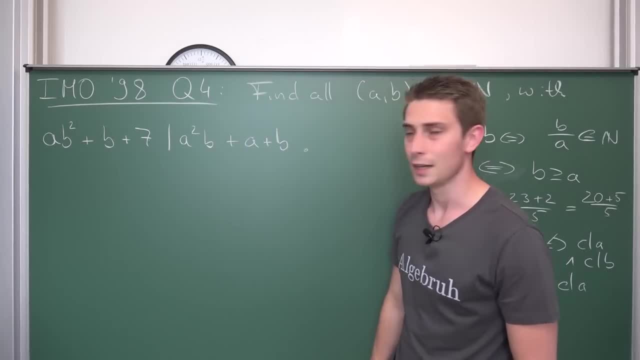 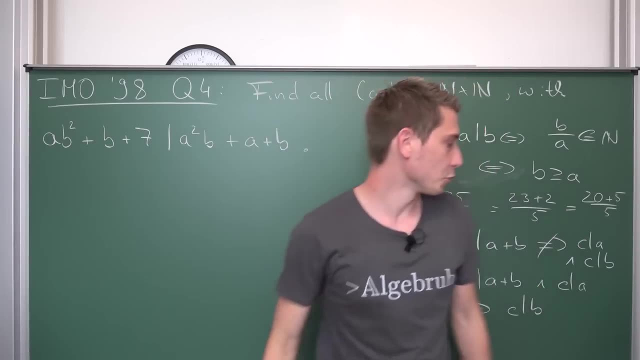 Well, here's a B squared missing. Okay, This sucks, All right. So, in the first place, we are missing a B squared here, what we have here, and there's one more property for the division that We could make use of, namely if we have a divides B. 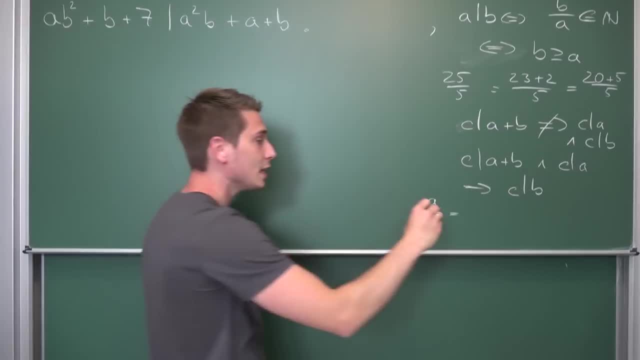 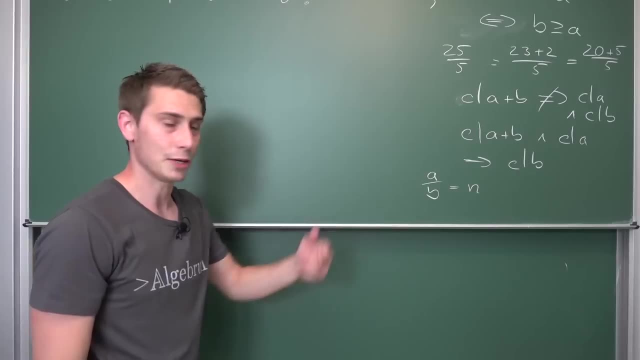 Then we can also say that this thing is element of n, meaning it's just some n element of n. Now, what we can do, we can multiply both sides by some non-zero element of n, Let's say M, R, for example R on both sides. Then we have something out of N. 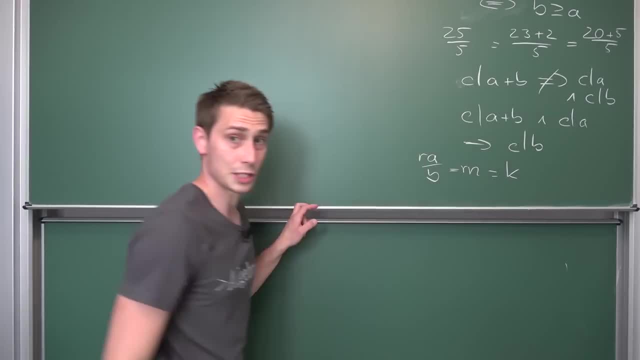 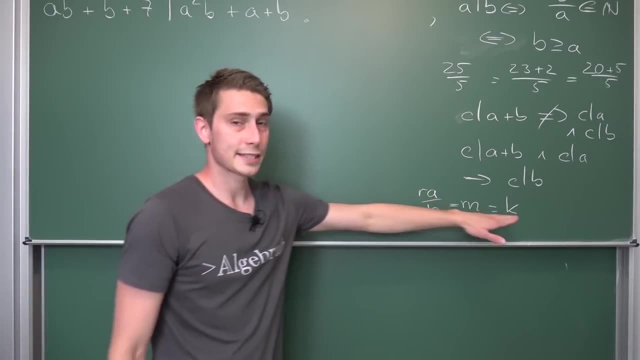 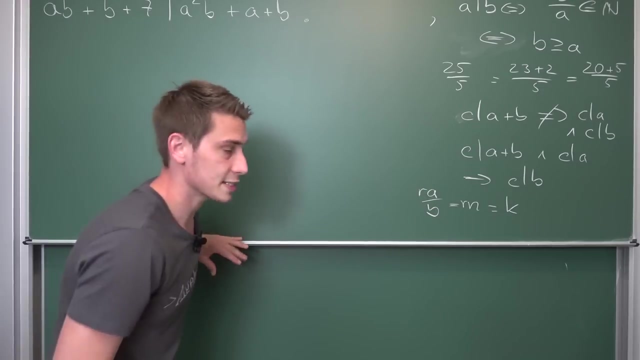 Times something out of n is yet again element of the positive integers, in our case meaning. what this means is we have multiplied both sides by a certain factor and it's still an n. meaning our B still divides a R times a, even though it divided a in the first place. meaning what we can do here is: 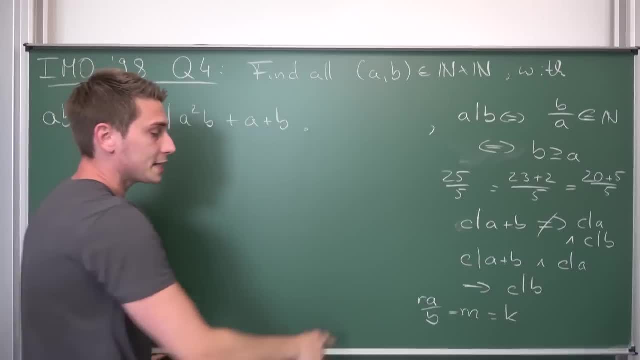 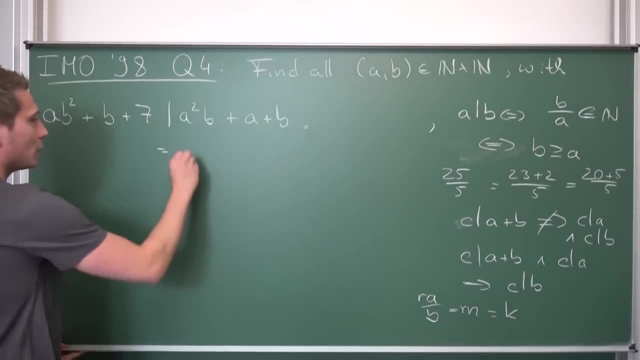 We can multiply what we have here in the numerator by some R and we are going to call this R exactly B, because we need a B squared here. I hope you can follow me meaning: we are going to multiply B by this whole expression, giving us a squared times B squared. 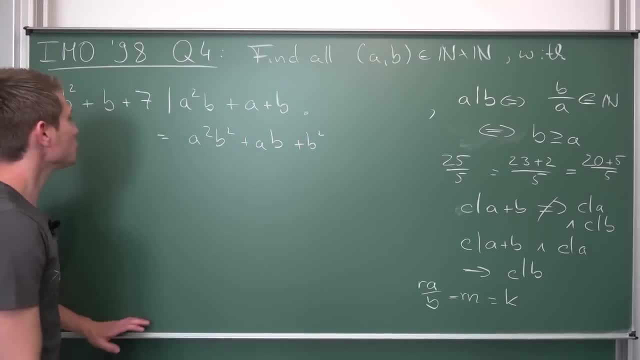 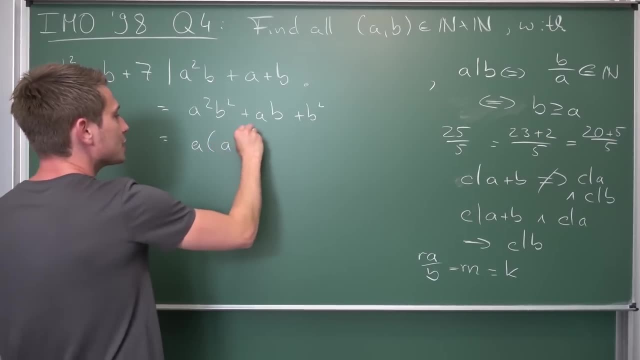 plus a B, Plus B squared, and this is good, right, Because now we have a times B squared. This is what we have here. All we need to do is check out the a meaning. This is a times a B squared plus well B, and then plus B squared. Ah, 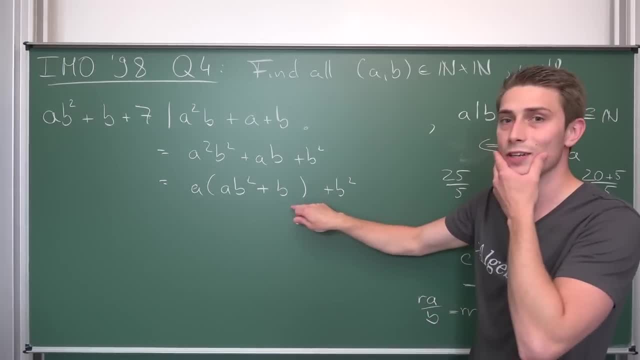 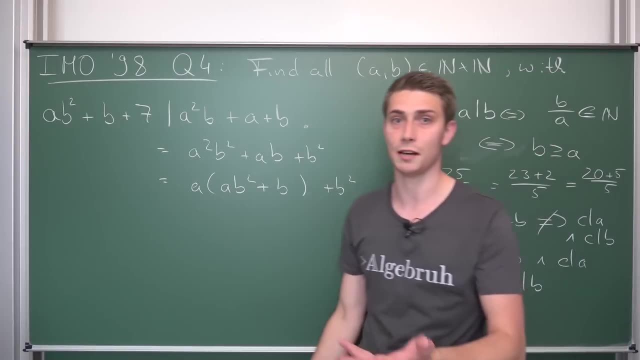 Shit, something's missing yet again. Our 7 is missing. Well, what can we do here? I mean, it really doesn't hurt us to add a 0 In here, so we can always add a 0 and it doesn't change anything if I place. 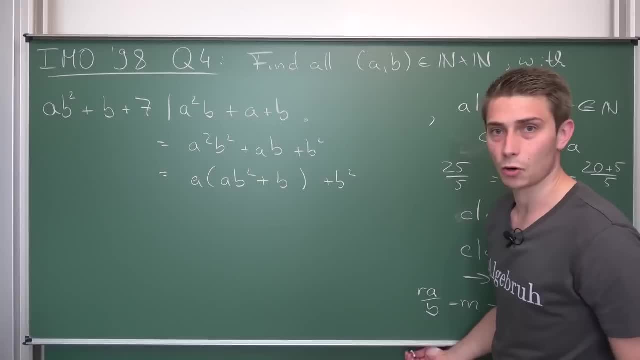 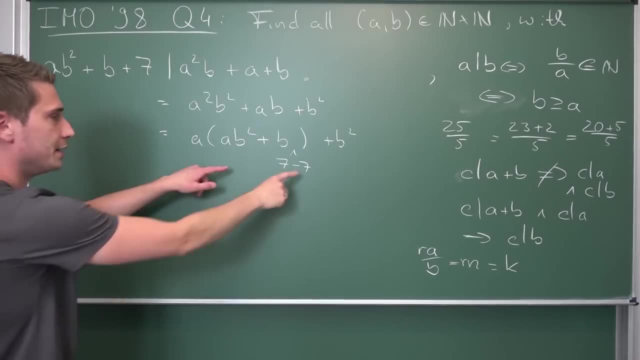 No, no other apples to a bunch of apples. you're still going to be left with your bunch of apples that you had in the first place. so let us add a 7 and subtract it yet again, and Negative 7 times a is something we can bring to the outside, meaning overall We are going to end up with a times a- B squared. 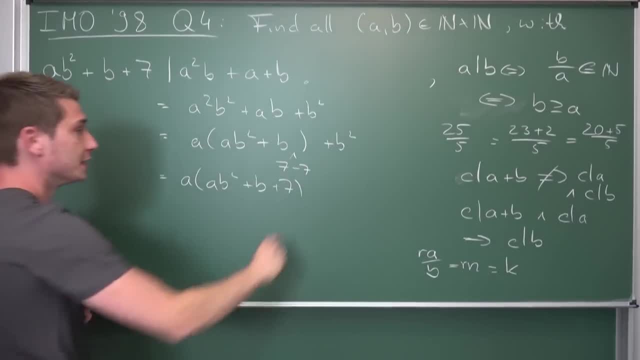 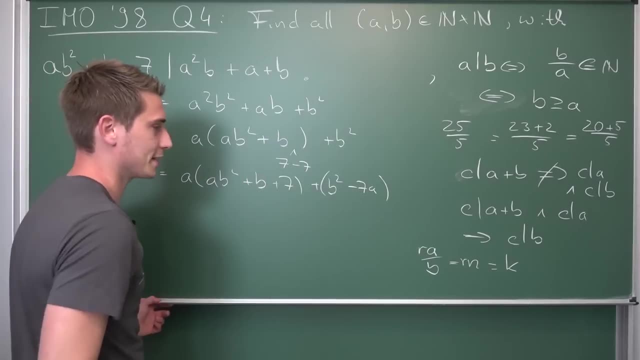 plus B plus 7, which is exactly what we have here, plus B squared minus 7a, which is exactly what we have here, plus B squared minus 7a, Which is this part that we have tracked to the outside. All right, this is good. 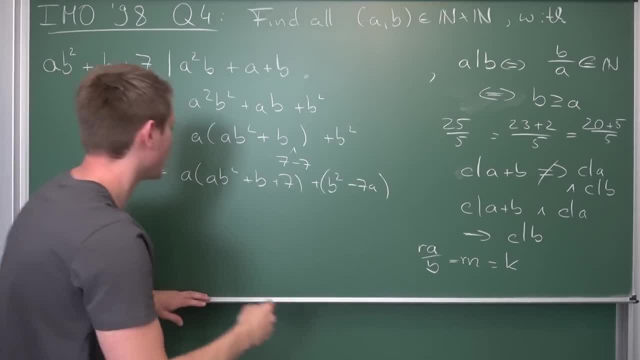 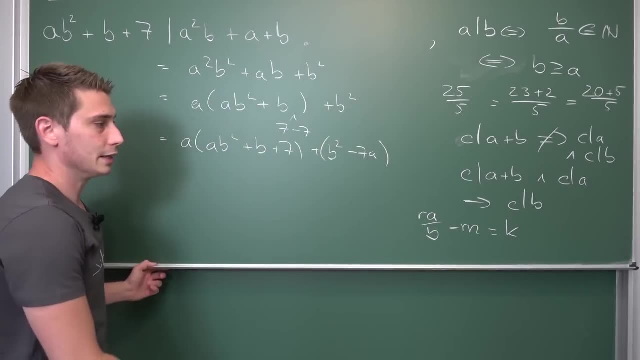 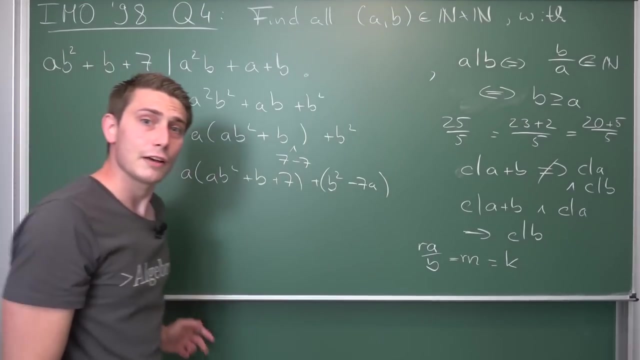 I mean, I'm obviously a. B squared plus B plus 7 gets divided by this factor, even though we have a here. But this is the same argumentation that we have here in On our hands. basically, a is just an element of n, meaning for this equation to hold, we can have: 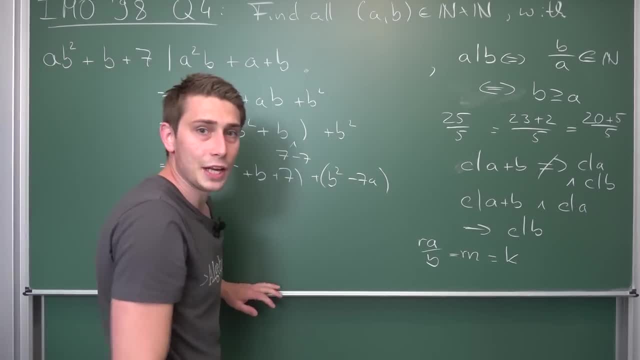 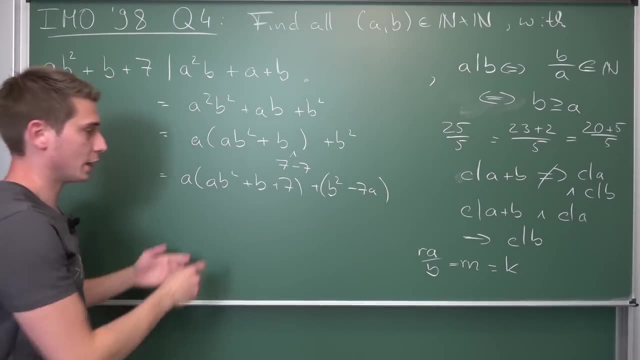 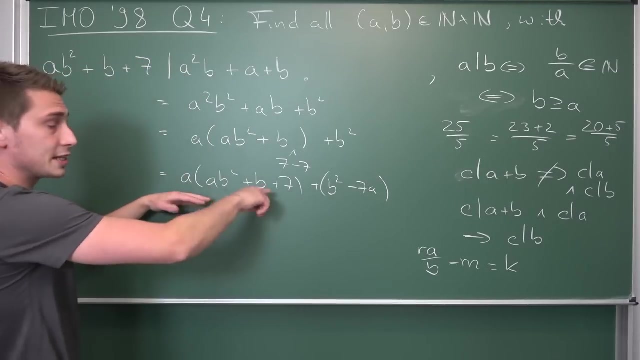 Two different cases at first. either B squared minus 7a is exactly 0, then this thing is identically equal to What we have here. it could happen probably for a being equal to 1- we don't know this yet- But if we have the case that B squared minus 7a is equal to 0, then this obviously gets divided by what we have here. 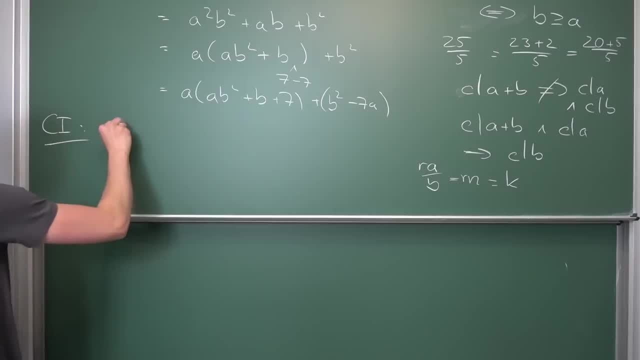 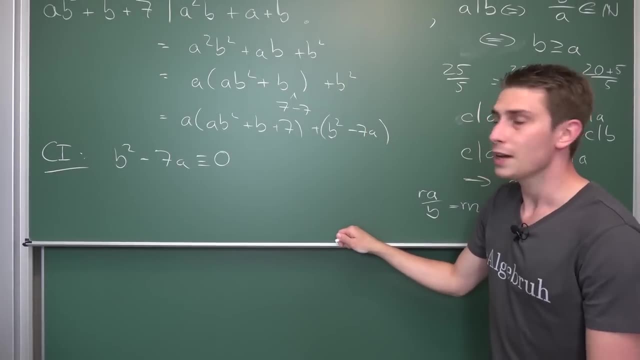 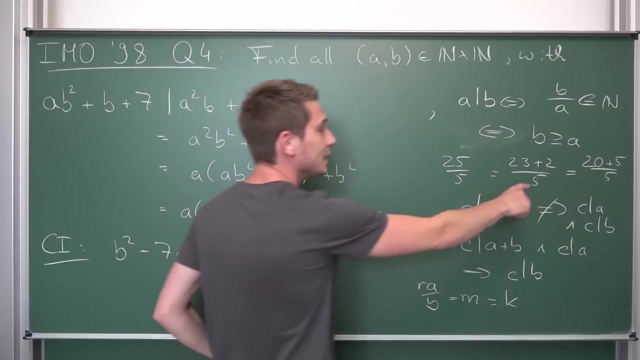 so the case 1 Is going to be that B squared minus 7a is equal to 0. this is a case that we can have. There's another case, though, namely that this part is non-zero Meaning. if this is non-zero, then we have the situation that we had here. 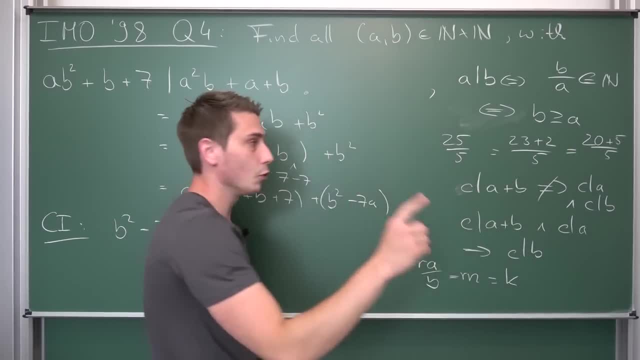 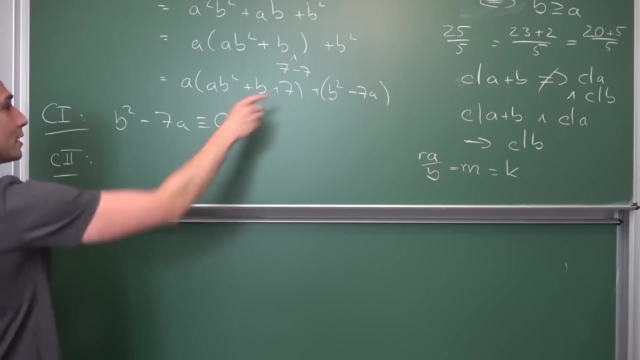 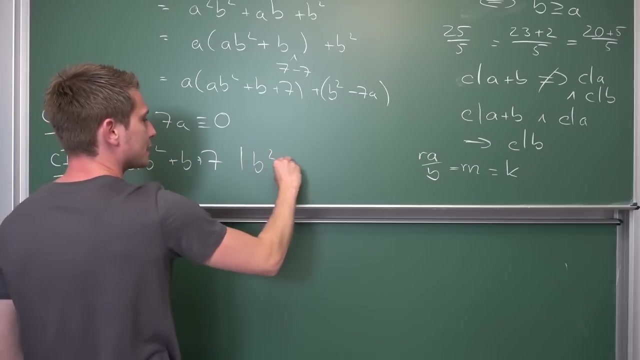 We had that 5 divided 20, but also 5 divided over 5 that we had up here. Okay, I hope you understand. so case number 2 Would mean that this factor up here, a B squared plus B plus 7, divides exactly our B squared. 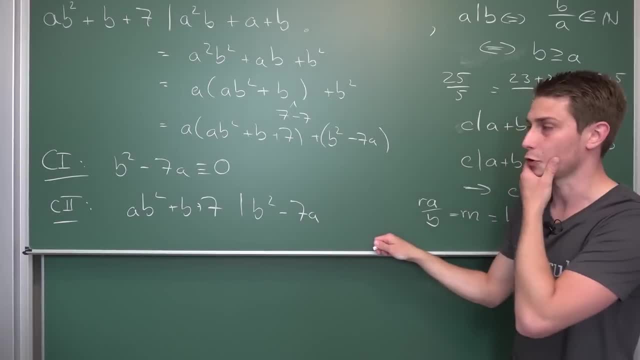 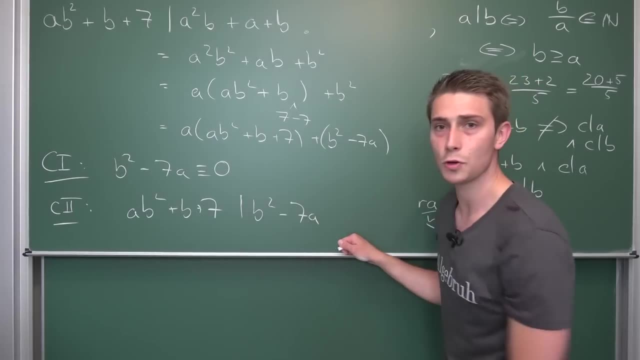 minus 7a. Alright, as far for those Explanations, how we got here and now we are going to go through the different cases and see how this turns out. Let us start with the first one, because it's easy. Let us add 7a on both sides. We can do this meaning for the case 1. 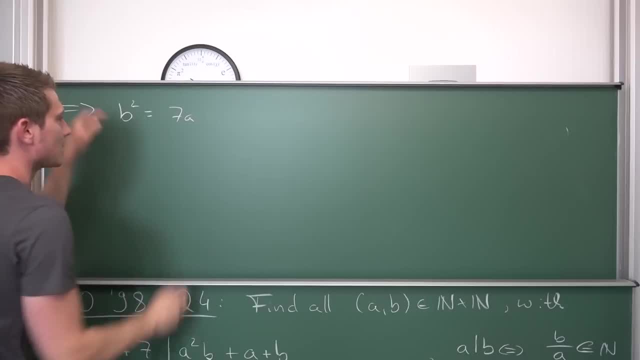 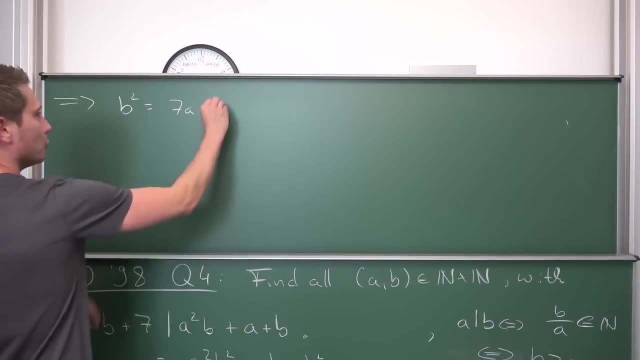 We are going to get that B squared is exactly 7 times a. now we can take the square root. I mean B must be positive. Okay, by this condition We're only going to take a look at the positive branch. Meaning B is does nothing but square root of 7a. 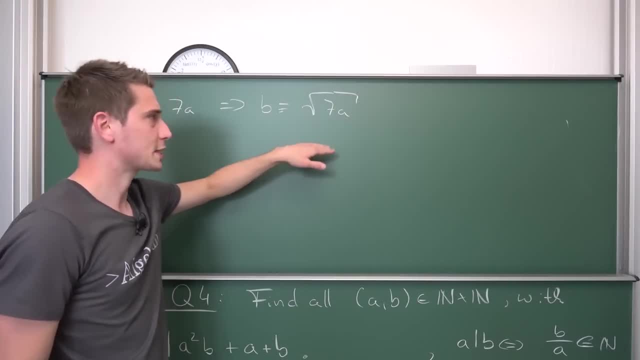 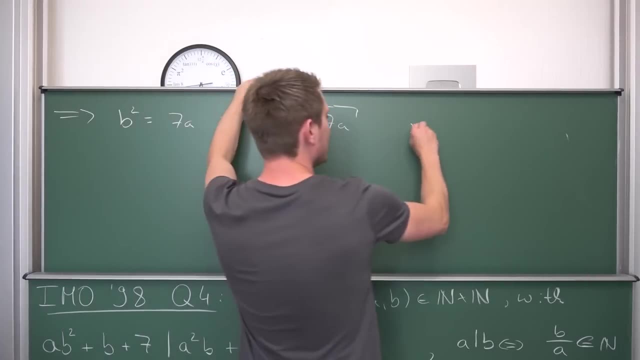 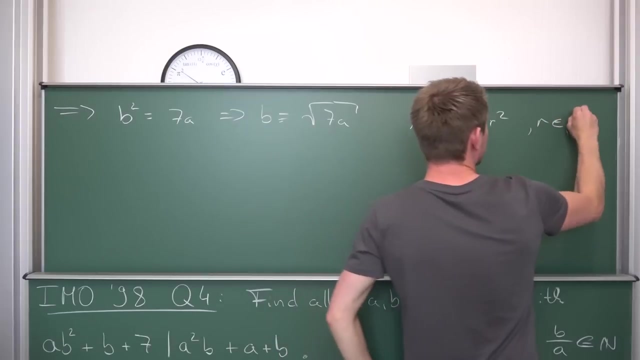 Meaning overall, we need 7a to be a perfect square, for B to be in n yet again. and there's an easy way to actually get this to be a perfect square, namely by choosing a to be equal to 7 times. I don't know. r squared where r is element of the positive and negative integers, because by squaring it, 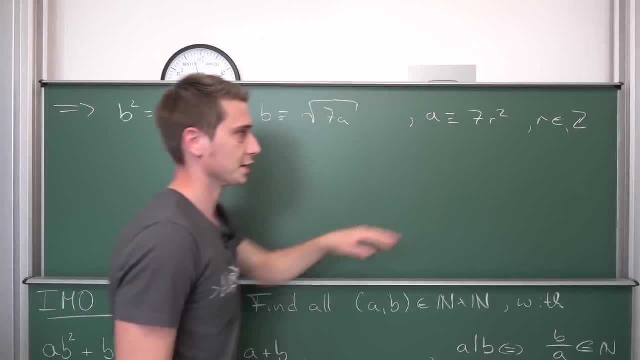 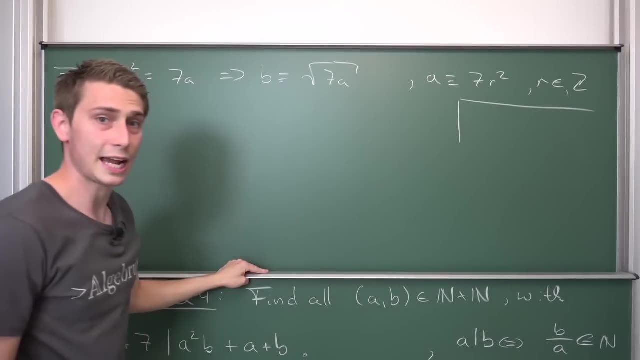 It really doesn't matter if we have a positive or negative sign here, meaning overall We have the set of infinitely many solutions. namely, the first solution that we can find by this first case is that our a and does not, and those must be ordered. pairs a and b are not symmetric here. 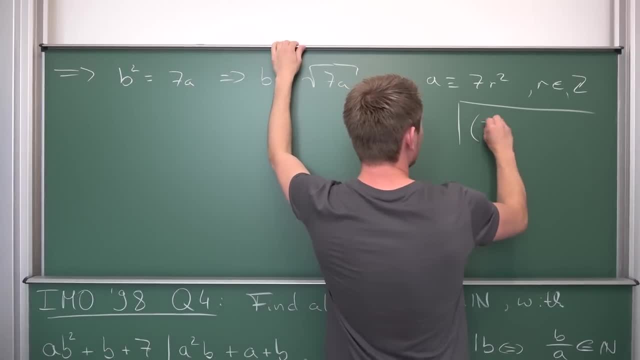 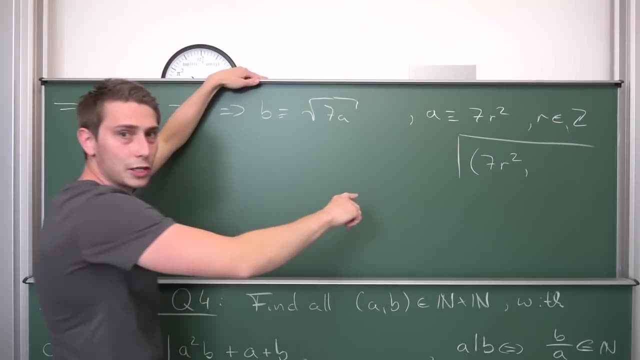 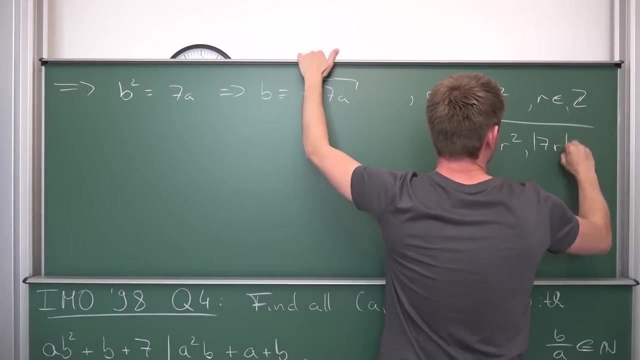 in our case, we are going to have a being equal to 7r squared, and Also we are going to have that B is does the square root of this meaning It's the absolute value of what we have here. So 7 times Well, the absolute value of r. basically so, the absolute value of 7r. 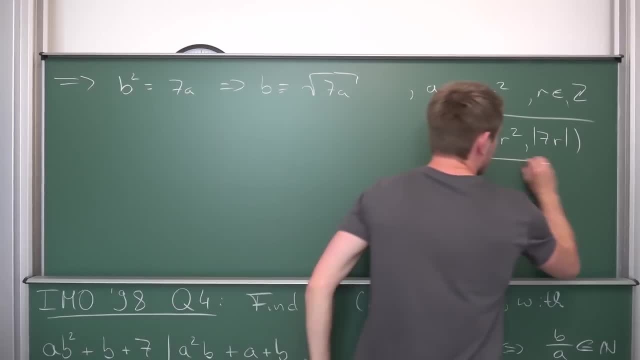 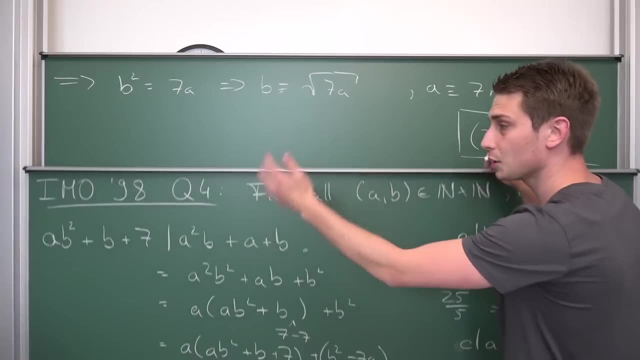 Obviously, where r is element of the positive and negative Integers. who so much talking here? I hope you could follow everything I did here. I just like explaining All the stuff for really, just because I don't like being like certain other people doing a lot of competitive math. 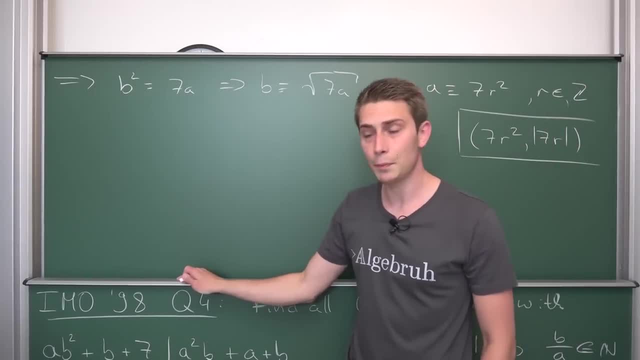 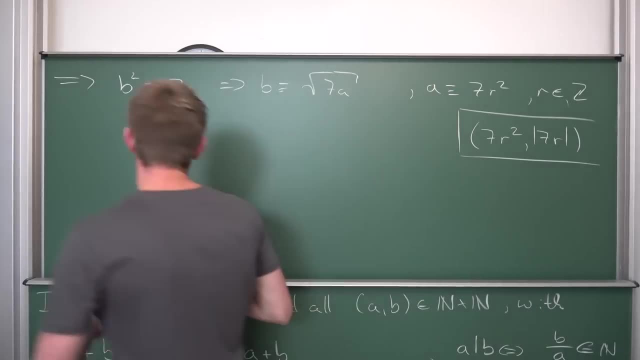 Content here on this platform and just assuming other people, the viewers, to have a 180 IQ. This is not something that I like. I actually like explaining each and every step such that there are no questions out there left. All right, now we are going to go through. 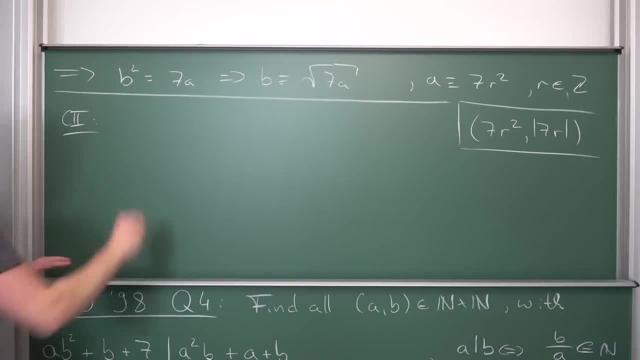 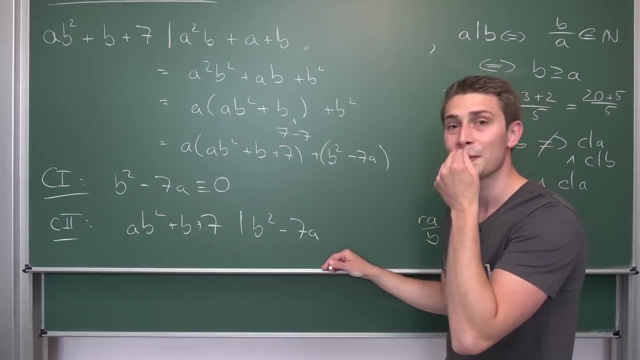 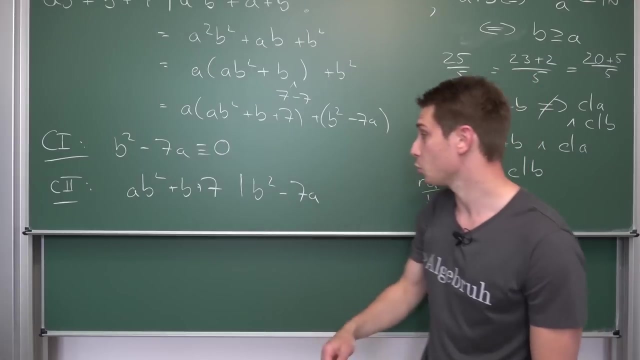 Unpopular opinion. here We are going to go through case number two. now for case number two, we have that b squared minus 7a gets the divided by this part, as we have here. but I could actually be two possibilities, because we are Subtracting 7a from this thing. for example, if B were equal to 1 and a is equal to 1, then we are going to get negative. 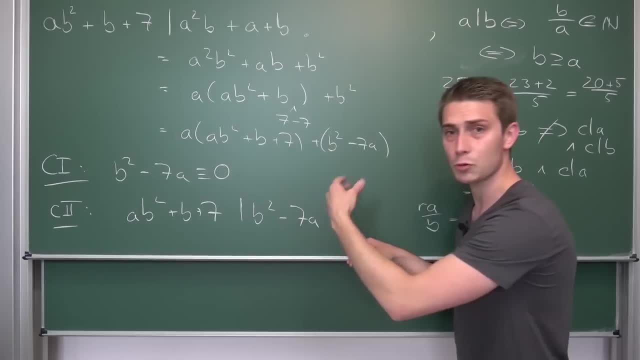 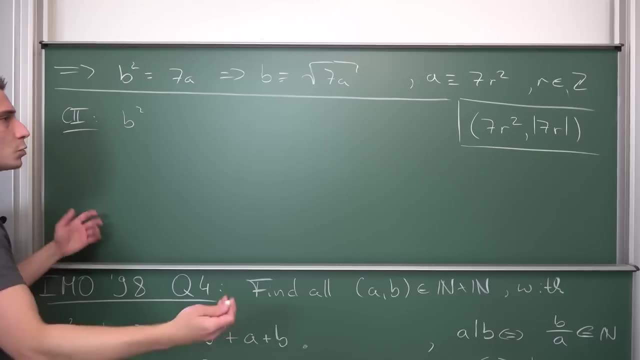 6, meaning one of the cases put could possibly be that b squared minus 7a is less than 0 or Greater than 0, doesn't matter. Which one are we going to start with, I don't know. b squared minus 7a. 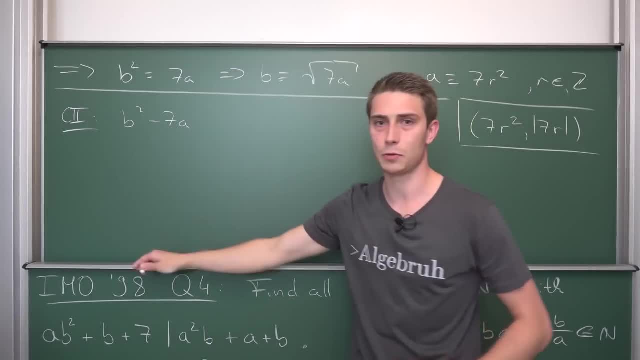 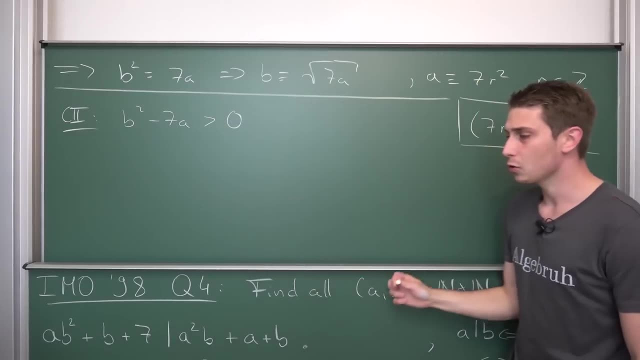 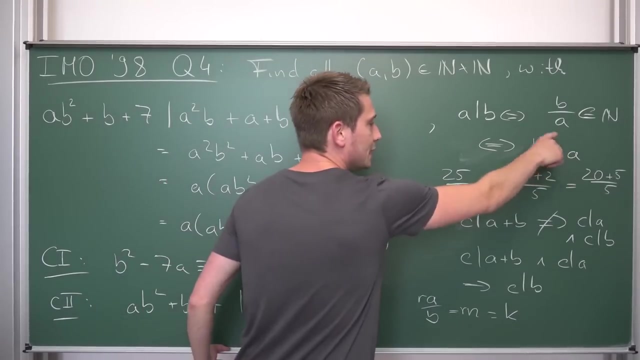 It could be greater than 0 if we have, for example, a being equal to 0 to 1 and b being equal to 3.. Okay, so greater than 0 in our case, and now we are going to see how that turns out. I mean, we still have this condition that I have said at the beginning. 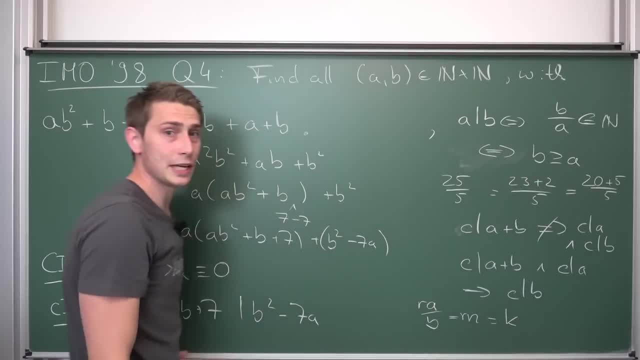 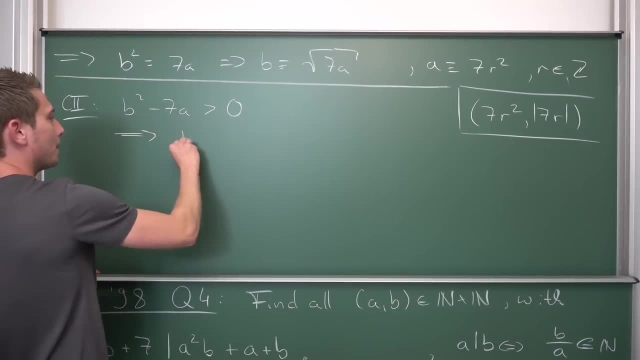 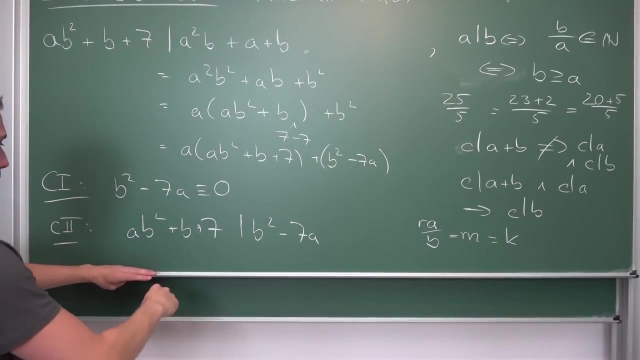 We need the numerator to be greater or equal than the denominator for something to be divided by another, something Meaning overall. we are going to have that our numerator, b squared minus 7a, must be greater or equal to our denominator, which is exactly this thing right here, ab. 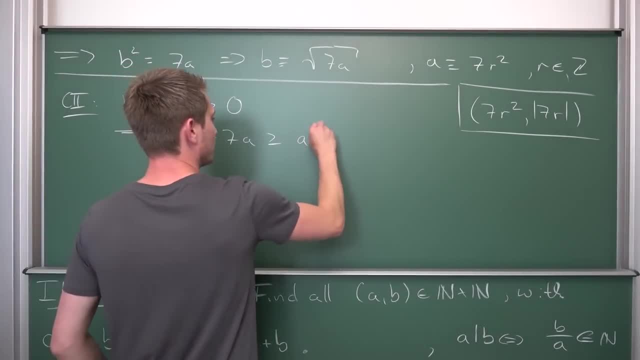 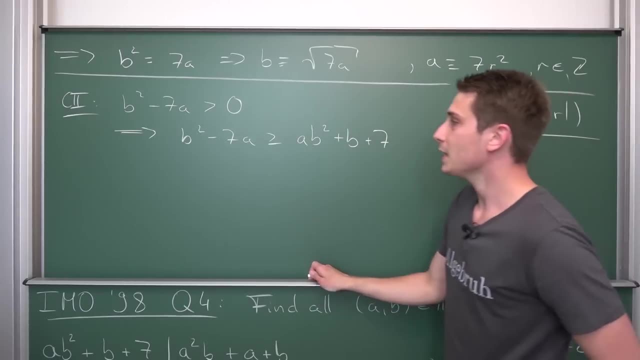 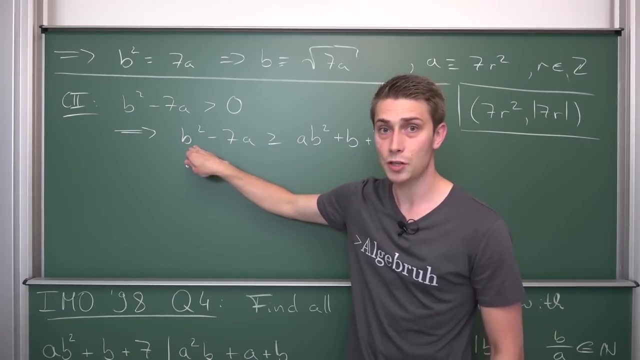 squared plus b plus 7.. And now we are going to well play around with this expression a tiny little bit. I mean our b squared that we have here. our b squared minus 7a is obviously strictly less than b squared, because just because a is strictly positive, meaning we are always going to have a greater or equal to b squared minus 7a. So we are going to have a greater or equal to b squared minus 7a. So we are going to have a greater or equal to b squared minus 7a. So we are going to subtract something from b squared meaning. 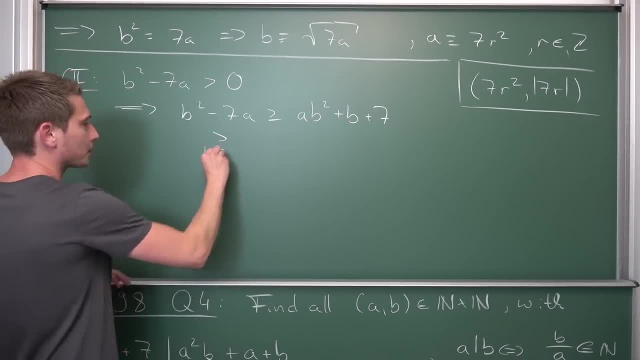 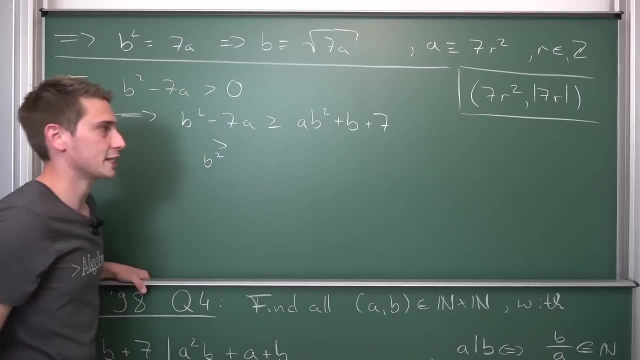 what we have here, this part is strictly less than b squared, But, on the other hand, what we have here is that b squared is strictly less than what we have here, actually, because, well, a is positive. so we are scaling something up by something greater or equal to 1 already. 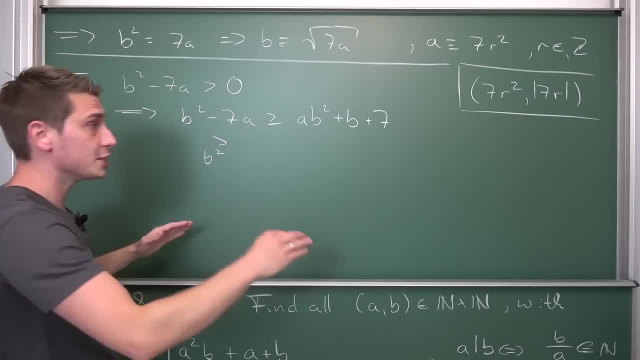 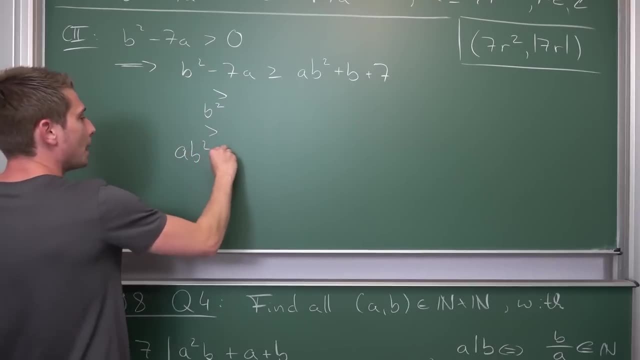 meaning ab squared is going to overtake b squared in each and every case, because we also have a b and a 7 in here, Meaning overall this is also strictly greater than ab squared plus b plus 7.. And what we are basically saying now is that 3 is strictly greater than. 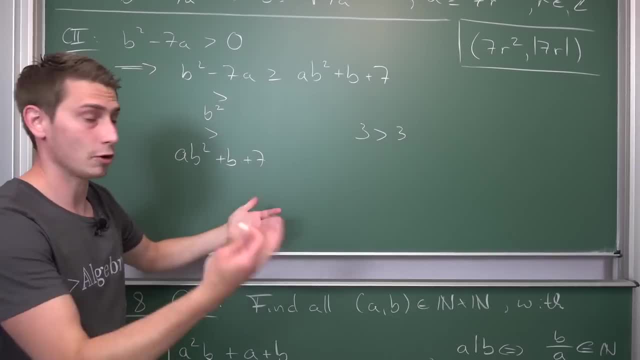 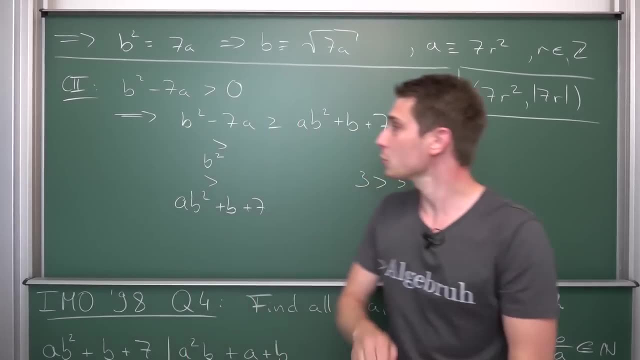 3, which doesn't make any freaking sense in the sense of total order relations. So this doesn't work out. that's a contradiction, meaning this case sucks balls. and now we are going to take a look at the case where b, squared minus 7a, is less than 0, and then we are basically: 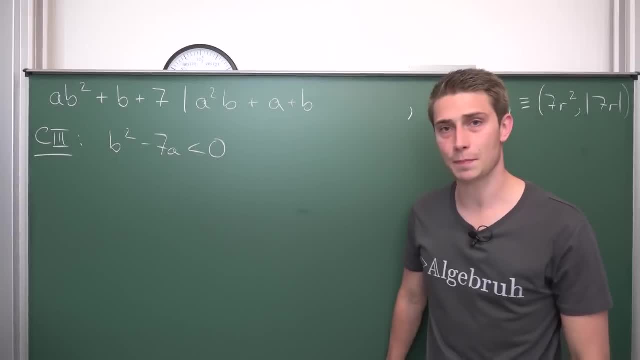 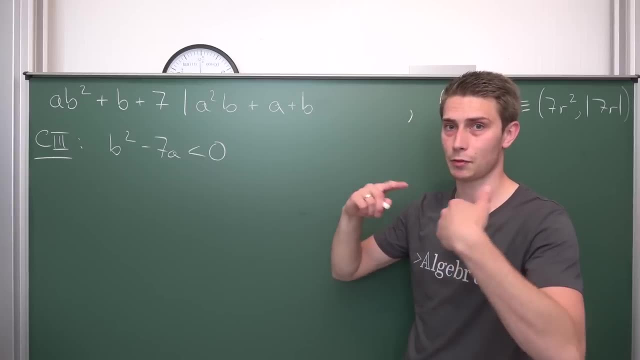 done. Now let us go ahead and get started. So b squared minus 7a is less than 0, meaning we can multiply both sides by negative 1.. This is one of the logical equations. So we can do one of the logical steps to make everything positive yet again, implying overall negative. 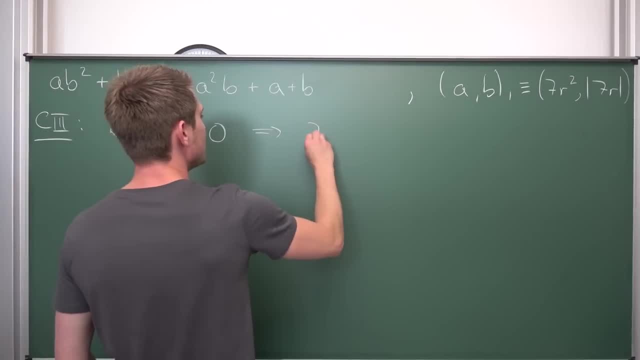 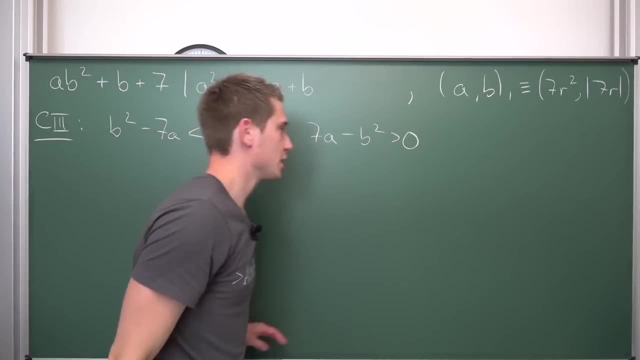 1 is not equal to 0, if you didn't know already. so we can multiply by it that 7a minus b squared is strictly greater than 0.. And now we can go by the same argumentation as before, Namely: 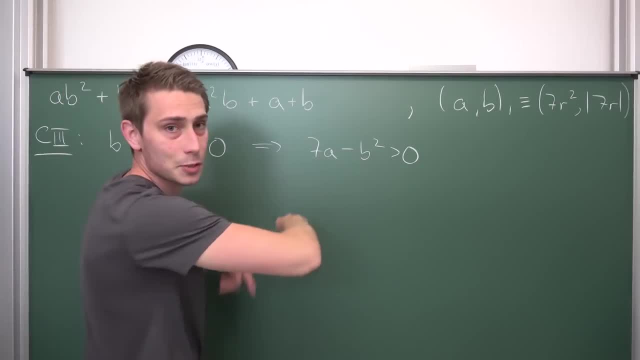 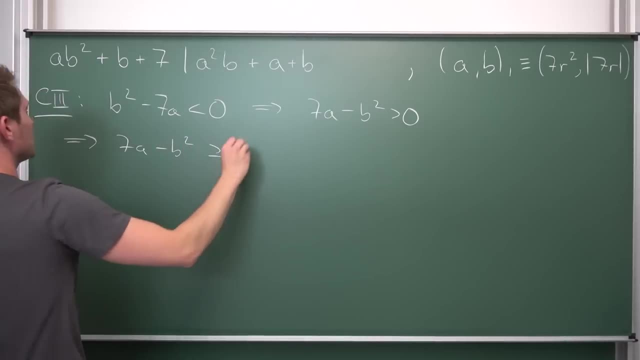 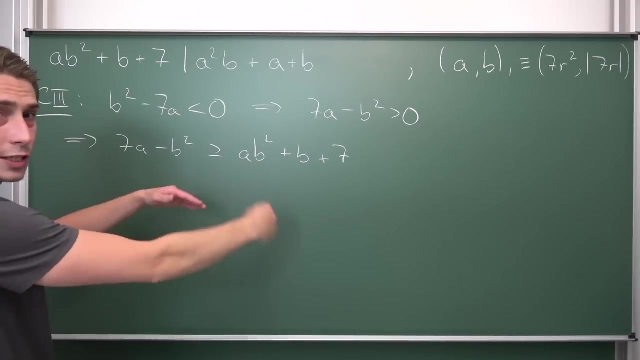 this term divides 7a minus b squared. meaning 7a minus b squared is greater or equal to what we have here. Meaning 7a minus b squared is greater or equal to ab squared plus b plus 7. and now we are going to go ahead and solve the time a little bit for a and b respectively on the sides. so 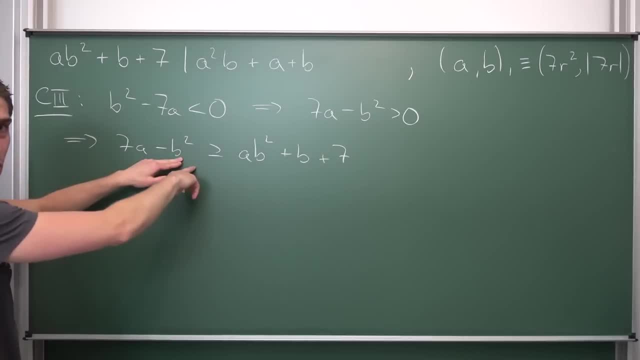 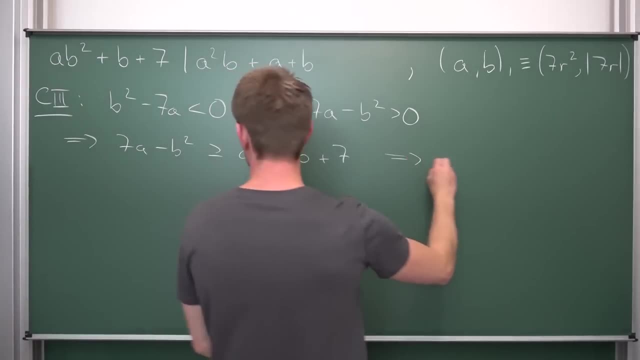 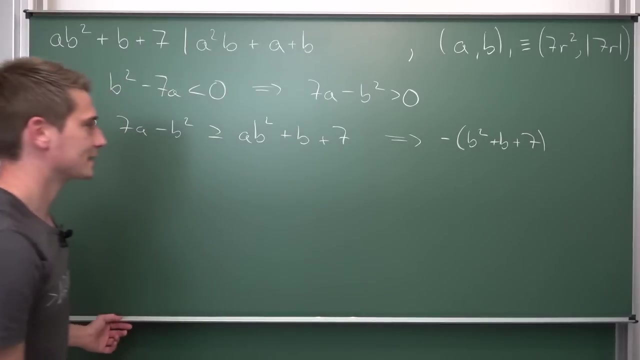 We are going to subtract b on both sides and 7 on both sides, leaving us here with negative b squared minus b minus 7. Factoring out the negative, it's going to leave us with negative b squared Plus b plus 7.. I hope you can see where this came from. Okay, just some. 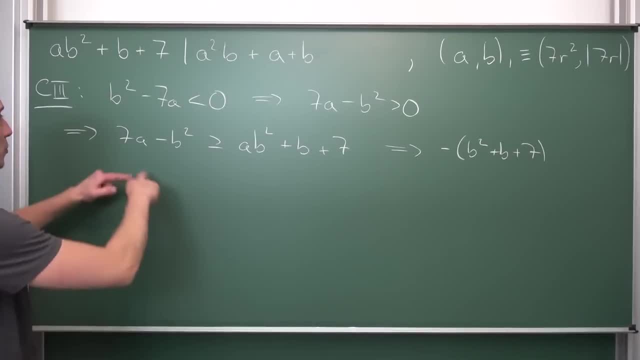 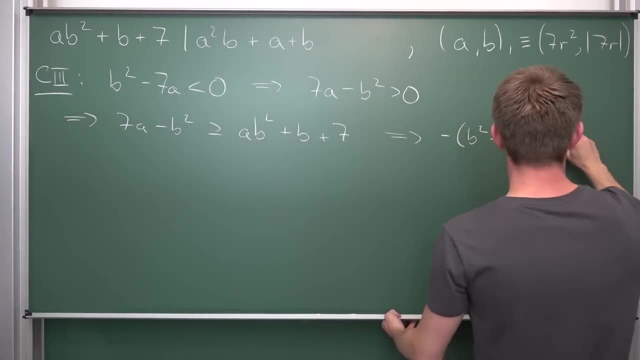 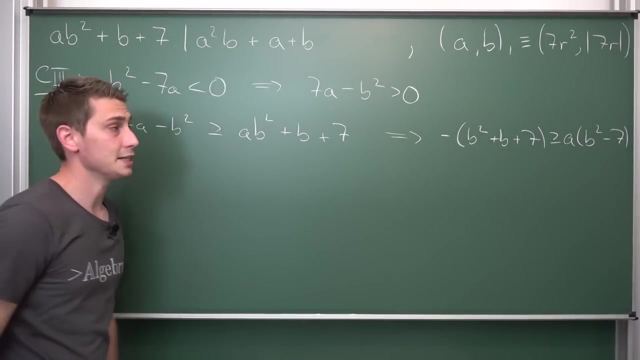 First-class mental arithmetic here. and then we are going to subtract 7, a on both sides and factoring out the a, Meaning this is greater or equal to Exactly a times b squared minus 7. The reason why I split it up like this is b squared and b and 7- they are all positive, meaning this side right here. 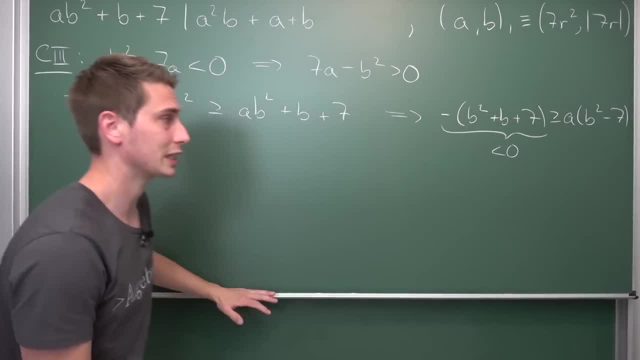 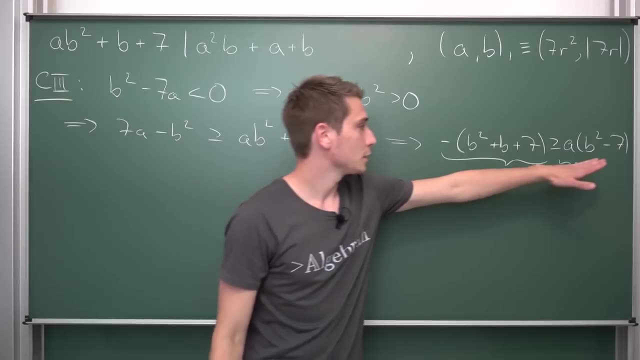 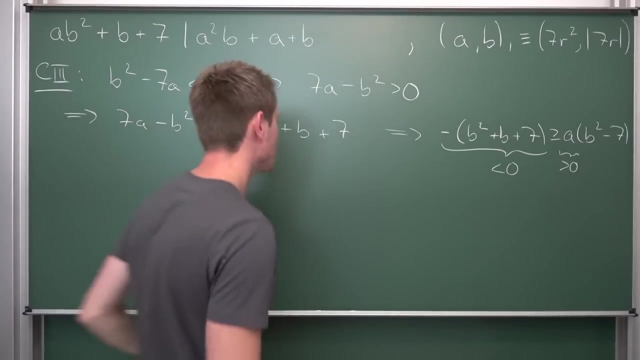 is obviously Less than 0, strictly less than 0. a, on the other hand, is positive, Greater than 0, meaning to get To a negative number on this side, We must have that b squared minus 7 is less than 0, So this is one condition that we definitely need. 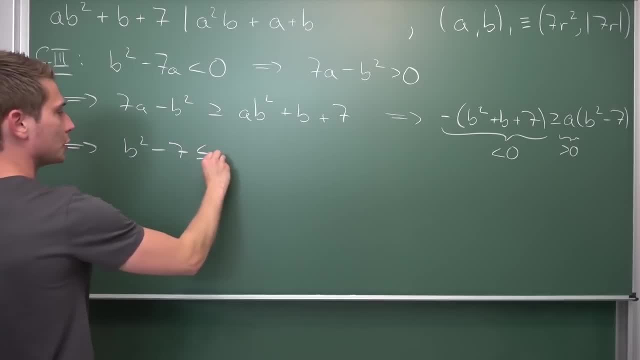 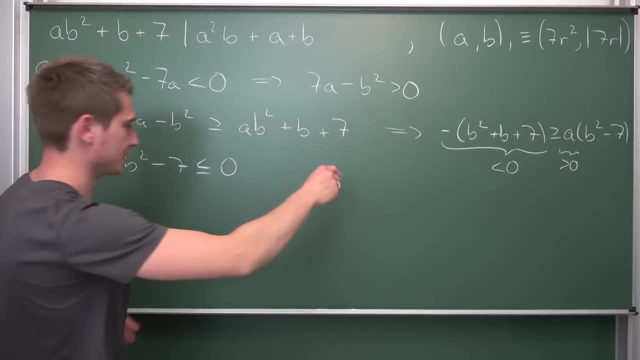 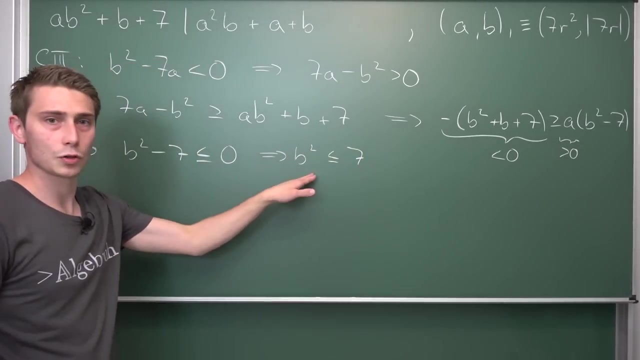 b squared minus 7 is Less or equal to 0. okay, This is something that we need in order for this order relation to hold. take a piece of paper, try it out for yourself. It's pretty easy to see. now we can solve for b squared. So b squared is thus less or equal to 7, and this only holds. 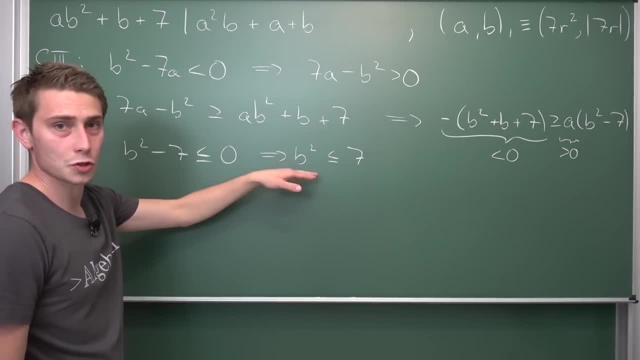 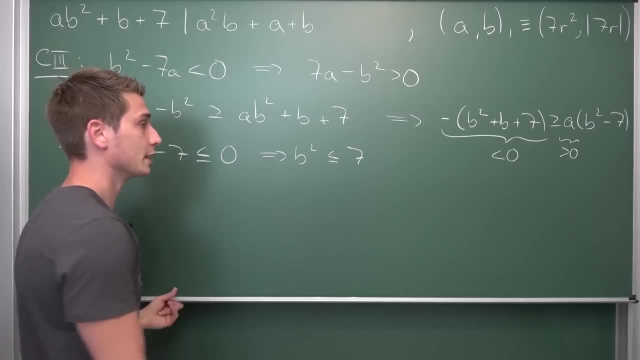 for two numbers for b, namely 1 and 2. so 1 squared is 1 is less or equal to 7 and 2 squared is 4 less or equal to 7 and 3 squared is greater than 7 already, meaning we can: 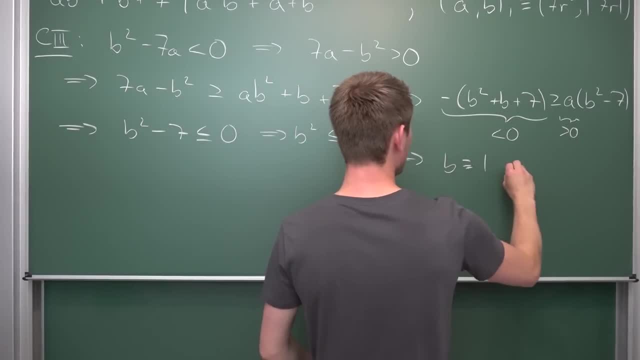 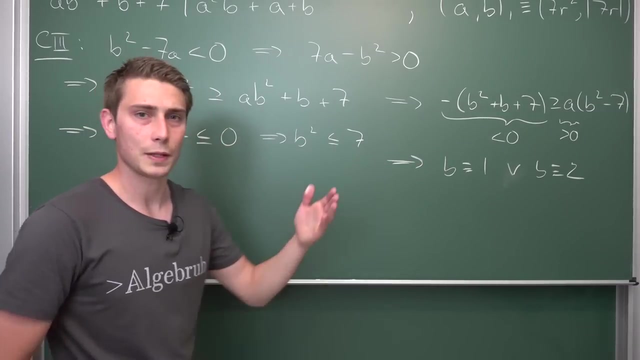 Conclude that b is either 1 or Yes, or b is 2 exactly, and also I did the wrong. This is why I erased it. Okay, have to think a lot what I'm doing here. now We can go through those two cases. There's going to be an outtake over on the second channel, flambeau maths 2, that you can. 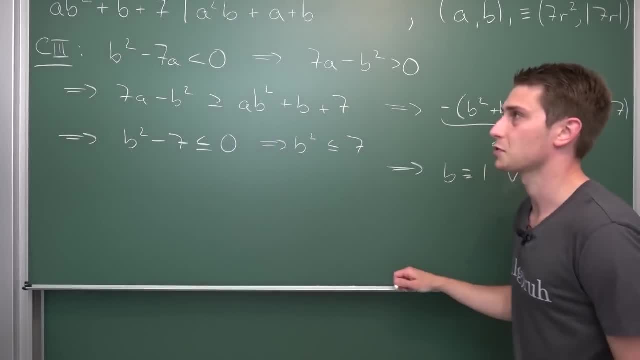 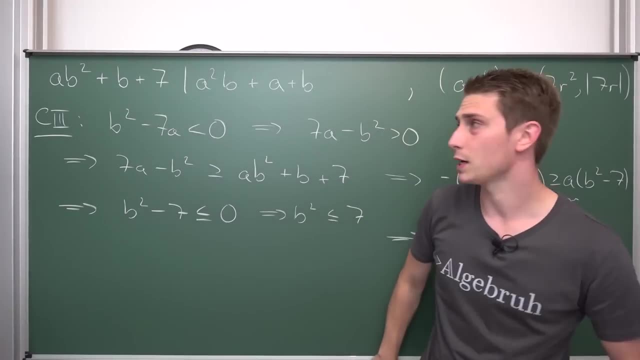 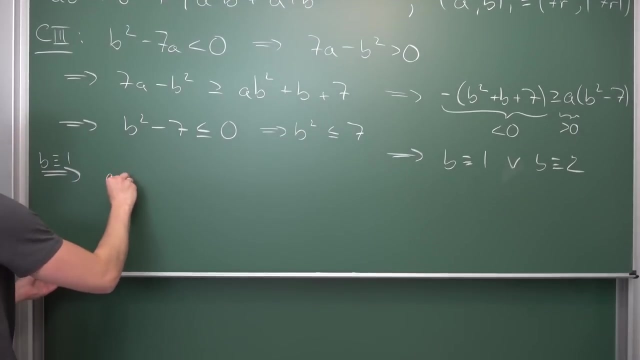 Take a look at later to see where the second stuff comes from, But the first leg us. let us take a look at the case where b is exactly equal to 1. We are going to plug it into here and see where this gets us. So, For b equal to 1, we are going to get okay, This is a plus 8. a plus 8, obviously. 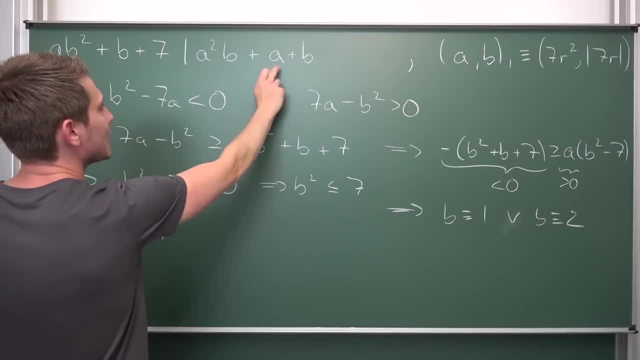 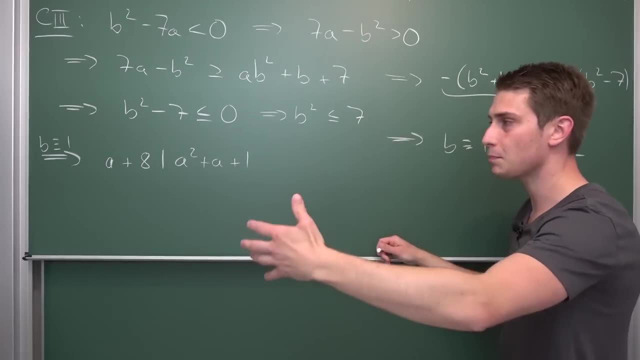 divides, in our case a squared plus a plus 1, and Now we are going to go through the same process that we did before. we are going to reduce it to something way easier. We are going to do it how we did it at the start of the video. 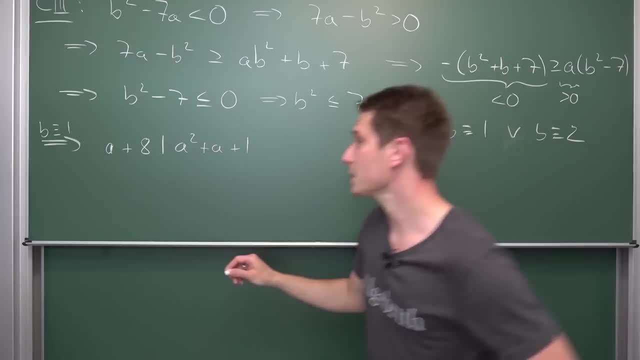 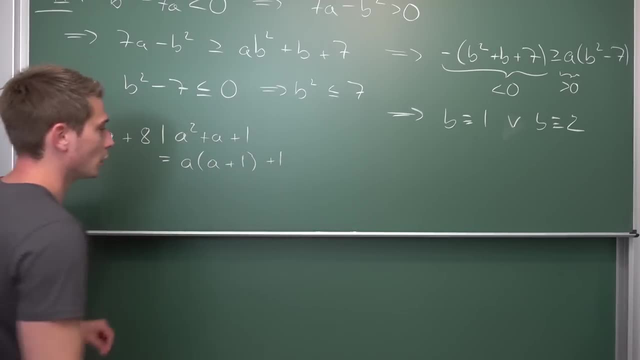 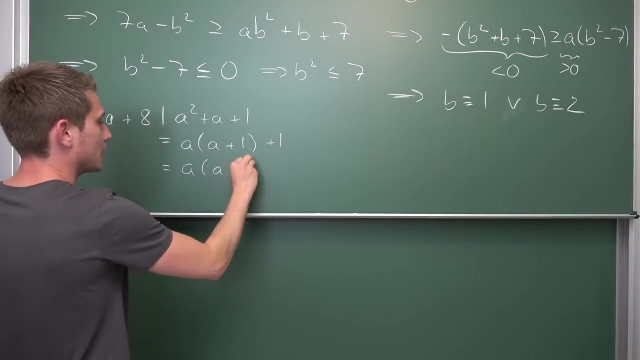 So we are going to bring this into the form of a plus 8 in some way, Meaning we are going to factor out the a here, So this is a times a plus 1 and the whole thing plus 1. we need a 7 here, so we are going to add a 7 and subtract it yet again, leaving us with a times a plus 8, and 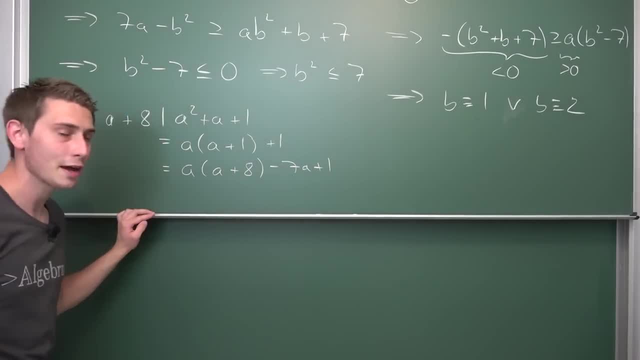 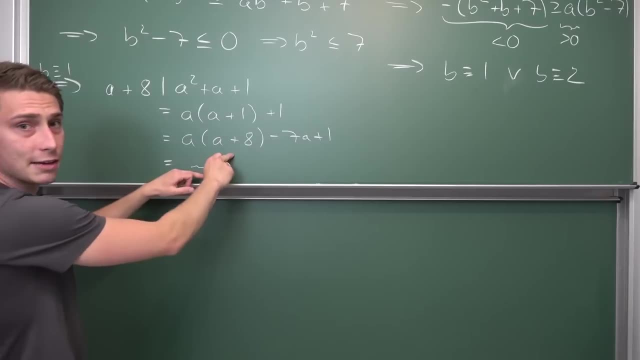 then negative 7a plus 1, and now here's where the magic is going to start. We are going to factor out the negative 7 here, so this is going to be something that is definitely divisible. We don't really care about this anymore. and then negative 7 times a. 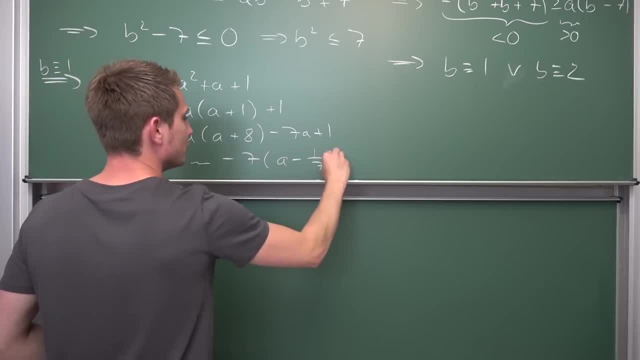 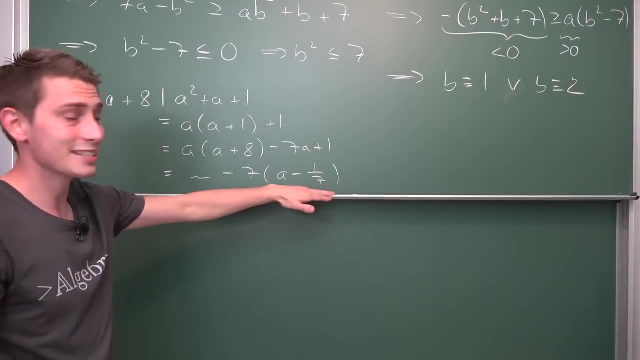 minus 1. seventh. Now we need to get to an 8 right here. We want to get to an 8 in some way, So we need to add and subtract Something in order for us to get an 8 in here yet again, to bring it into this form. 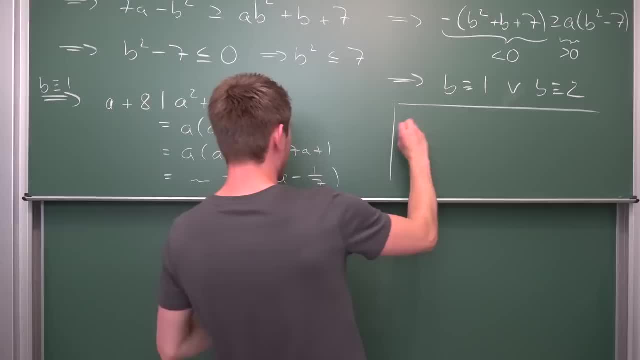 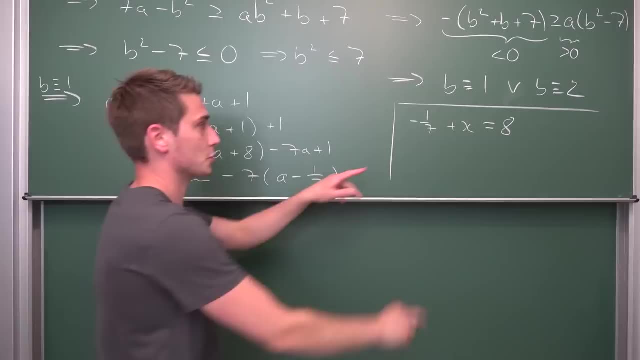 Meaning. what we are basically looking for is: what do we need to add to negative 1 7th, So plus X, to receive an 8? Well, this is pretty easy to solve. We are going to add 1- 7th on both sides. 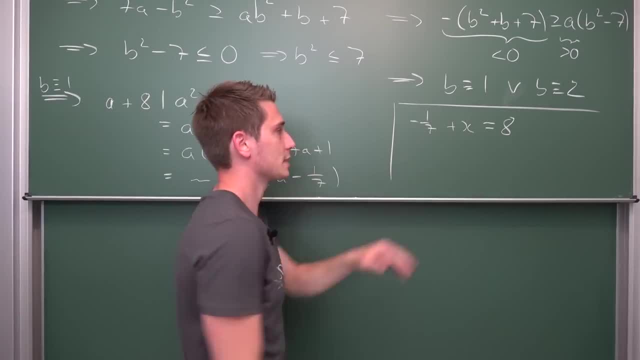 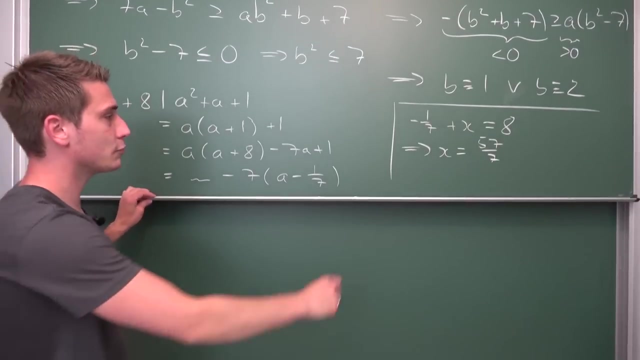 We are going to expand this thing by 7 over 7 is going to give us X being equal to 56 plus 1 over 7, so 57 over 7.. This is the Croton-Dick prime. Okay, meaning what we are going to get is if we plug positive 57 over 7 minus 57 over 7 into here. 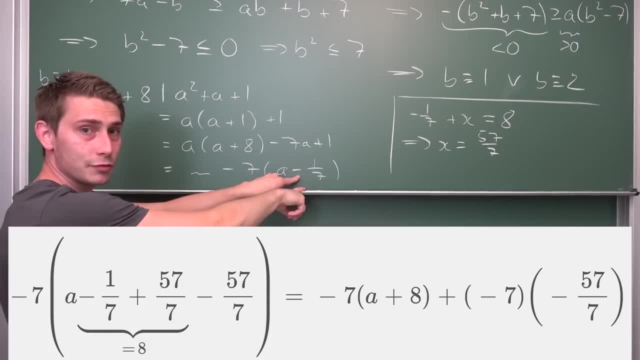 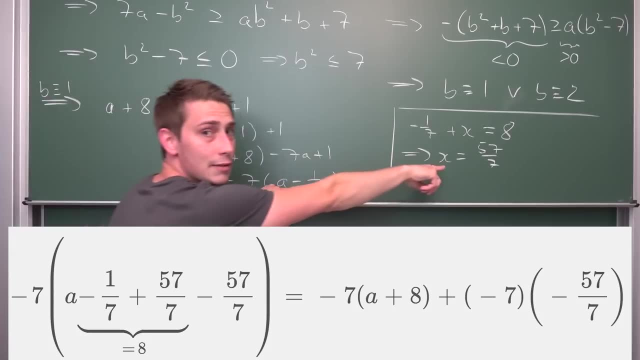 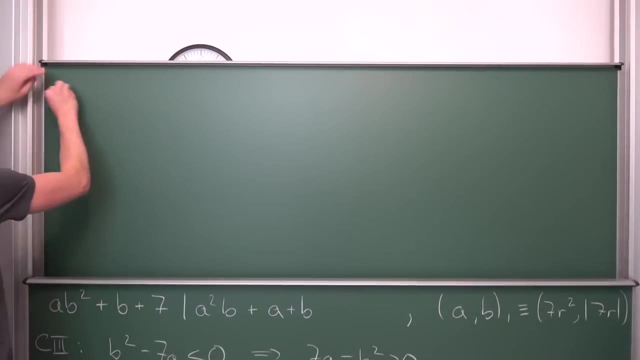 We are going to get exactly positive fifth, Yes, positive 8.. This is where we wanted to get, and then minus 57 over 7, which we are going to bring to the outside within a factor of negative 7, meaning overall. I Hope you could follow everything. Maybe there's an annotation there somewhere. 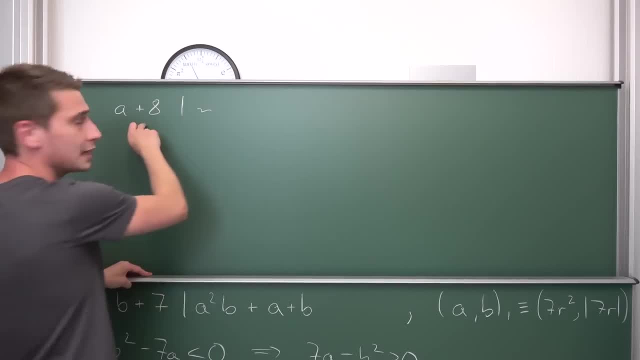 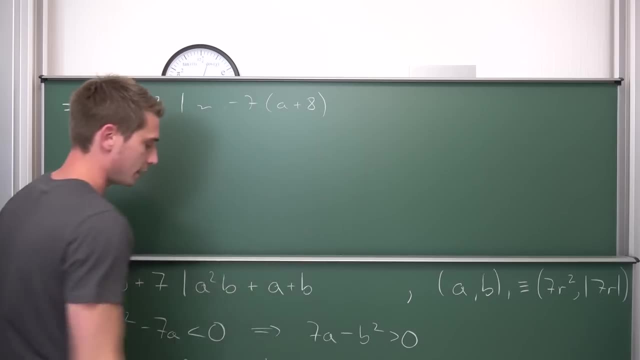 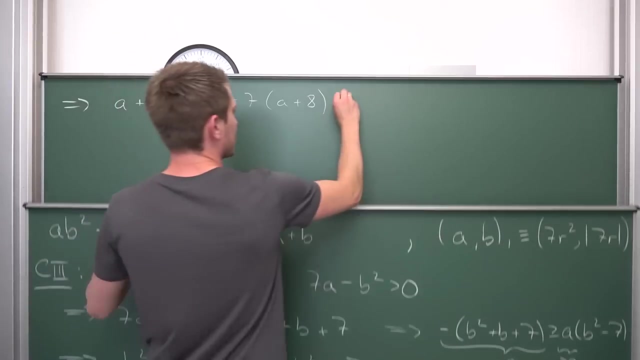 a plus a 8 is something that is divisible by a plus 8, obviously minus 7 times a plus 8. and then, like I said, negative 57 over 7. bring it to the outside, multiply it by negative 7 gives us exactly positive 57. this is divisible. this is divisible so by the first thing that we 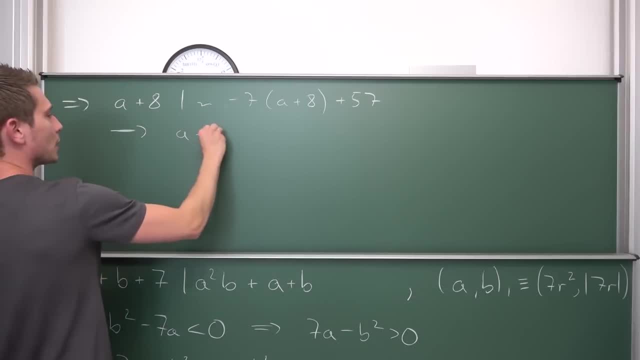 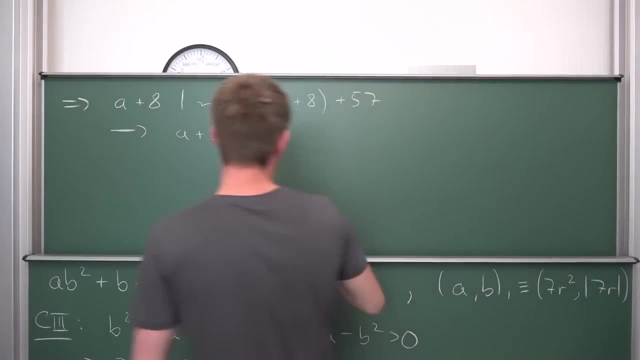 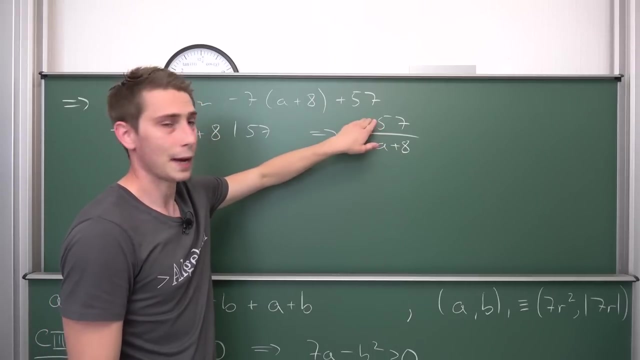 have stated in the video we have, that a plus 8 must divide 57. and well, now we can just go ahead and solve a fraction, basically just a little equation involving fractions. so 57 over a plus 8, this must be element of n, meaning our denominator is not allowed to surpass. 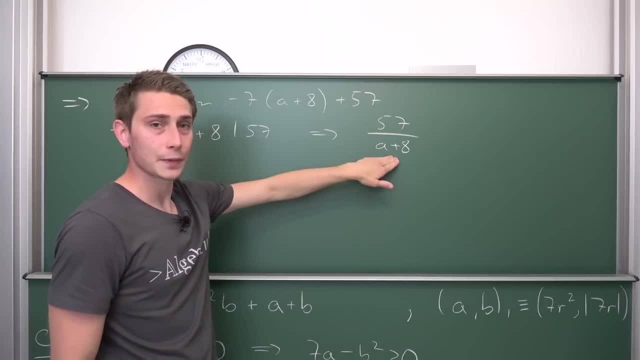 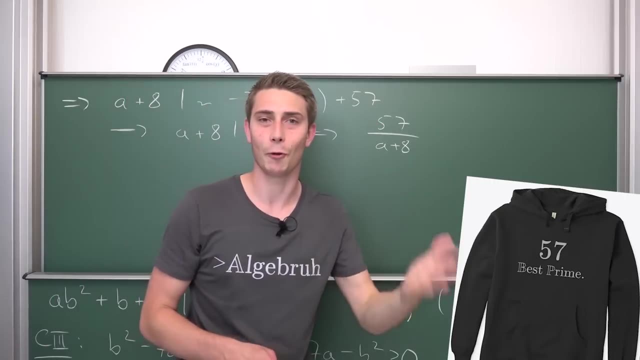 our numerator. so from the value, meaning a plus 8, must divide one of the prime factors up here. all right, so 57 is, by the way, the only prime that has more than two factors where, or has two factors where one is not equal to one. okay, 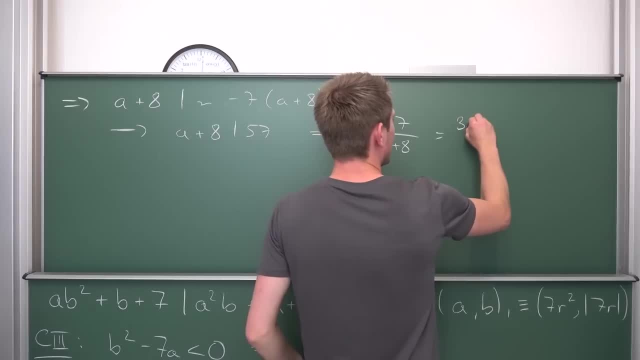 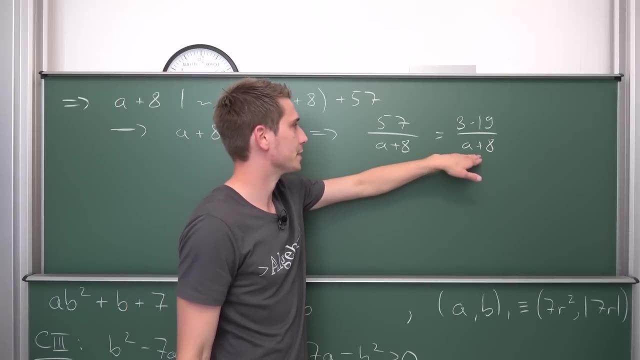 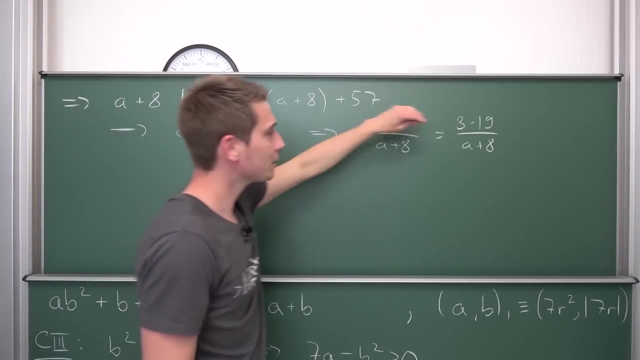 just a pretty cool fact: 57 is overall 3 times 19 over a plus 8, so obviously a plus 8 is greater than 3, so we don't care about that. so a plus 8 divides 19 or divides 57, meaning we can have: 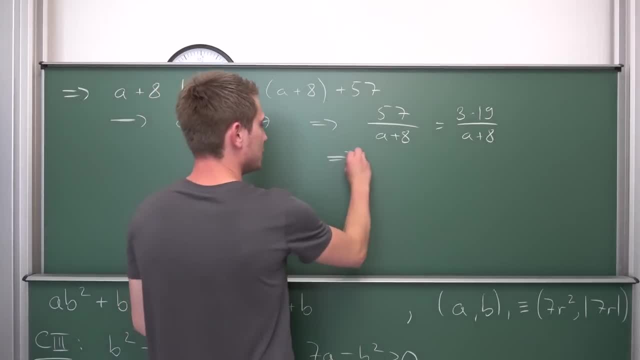 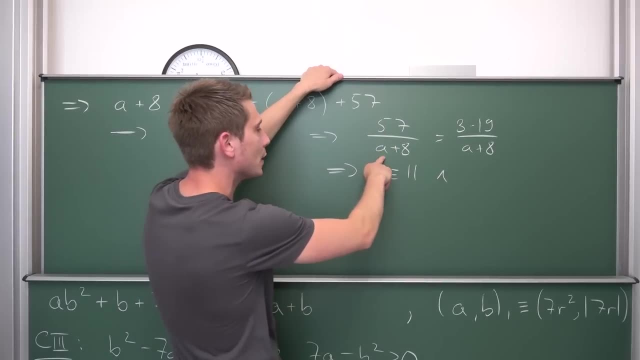 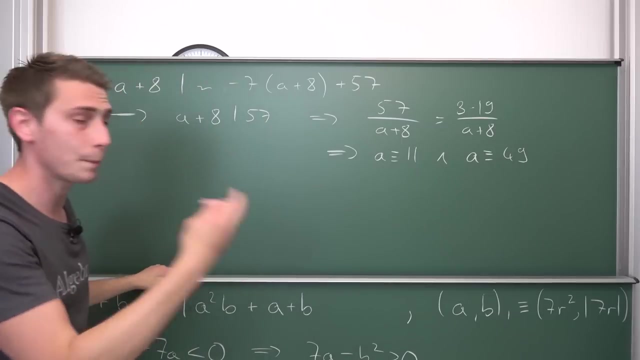 a being equal to 11, because 11 plus 8 is equal to 19, so a is equal to 11 and we have that a must be equal to. if it's 57, then we are going to have 49 plus 8 is going to be 57, meaning we have some more pairs at our hands, namely the next pairs: 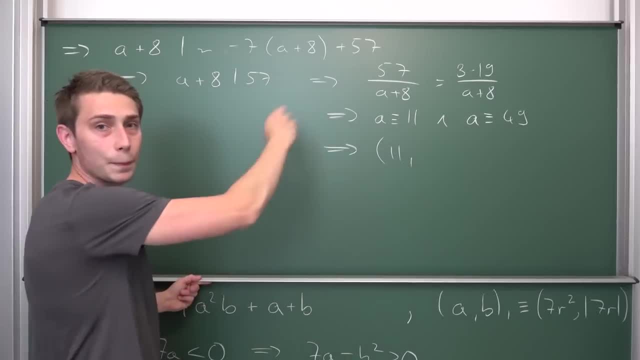 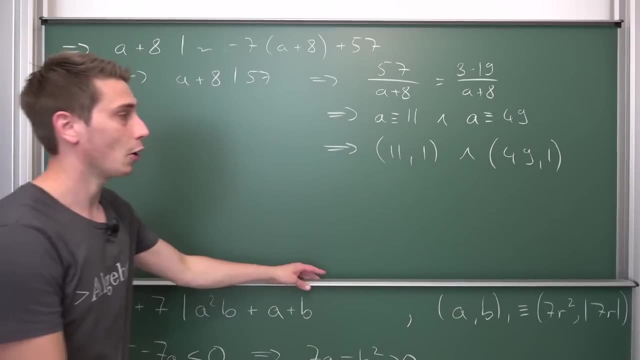 that we are going to get are exactly 11, and this was for b being equal to 1, 11 and 1, and we have the pair 49 and 1. All right, and now for the last case. so we are done with this, for B being equal to 2. 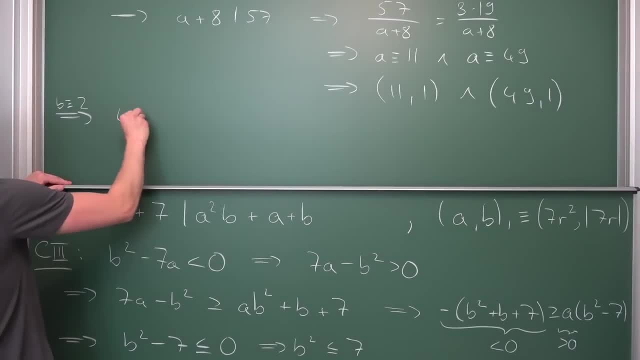 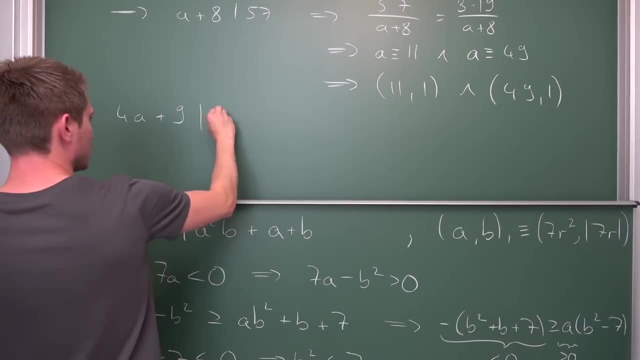 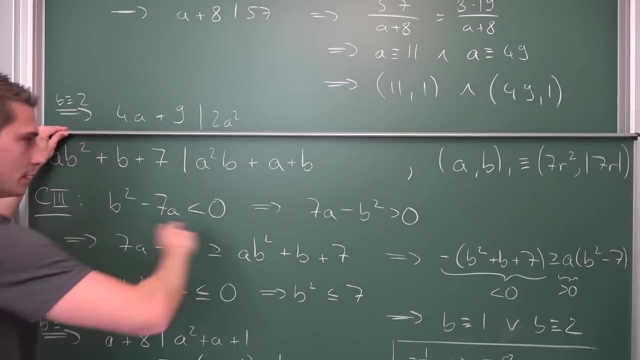 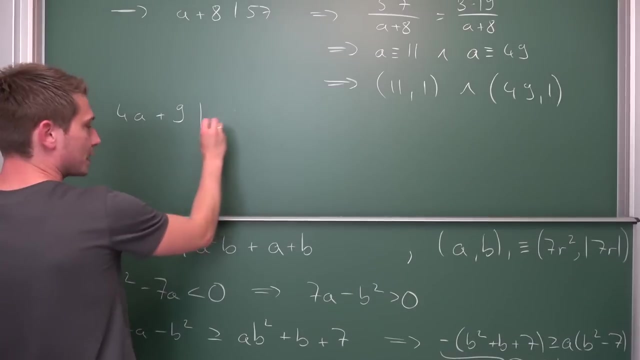 This gives us. let me plug this into here. we are going to get 4a plus 9 divides 2a squared Plus a. no, not this one, It has to divide what we have here. Sorry, I Mean it's the same statement, this one or this one right here from the division perspective. So 7a. 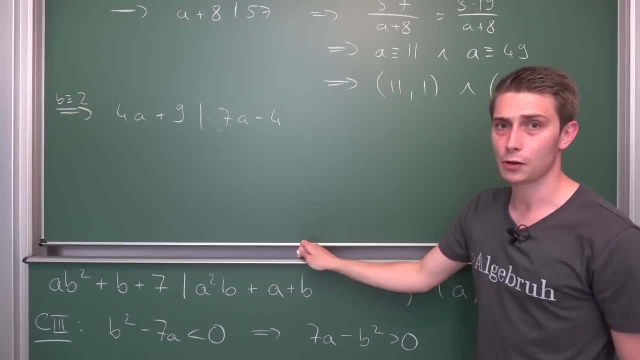 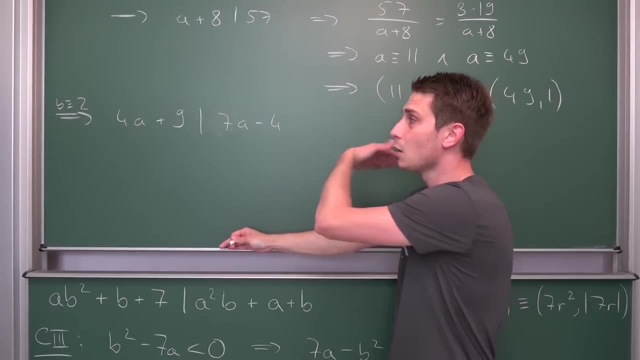 Minus 4 and, like I said before, there's going to be an outtake on the other video. There is no value for a in n that is going to satisfy this. if you want to take a look at What the solution to this one is going to be, take a look at papa flammy 2, because this video is already going on for long. 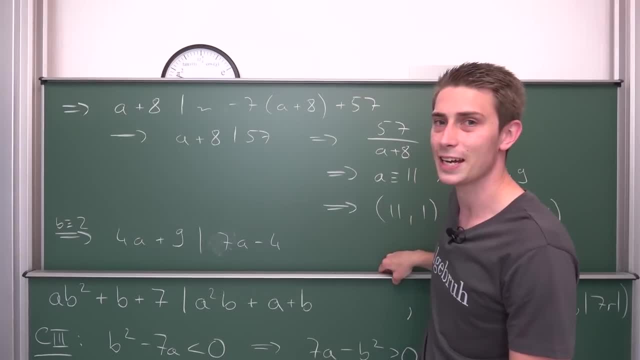 Enough. I thought that it's going to be quite a long video, So I don't want to harass you any longer, But if you are interested, link will be everywhere- info box, description, Etc. and I thank you guys for watching. I hope you did enjoy this video. 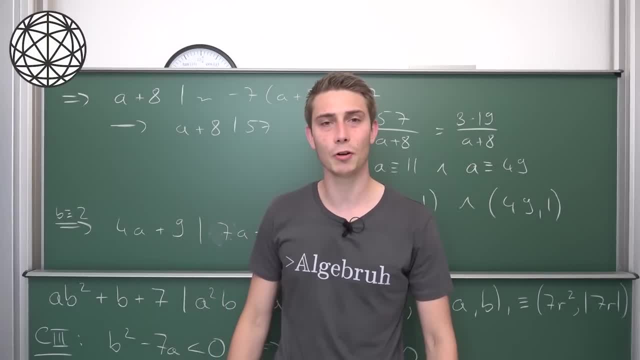 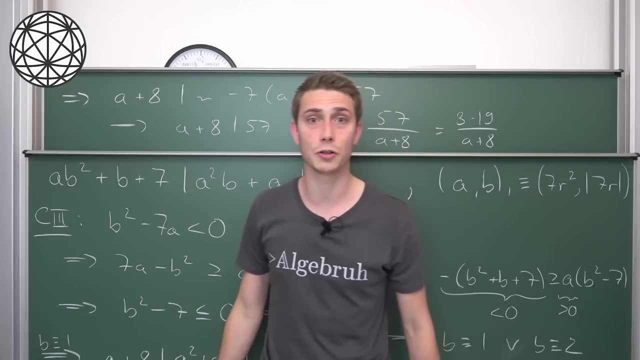 But before we end the video, I would like to thank today's sponsor, brilliant org, for sponsoring yet another video. They are honestly a lot of fun those compared to competitive math videos. And, yeah, brilliant does a really good job on Preparing you for competitive maths, So check them out Definitely. 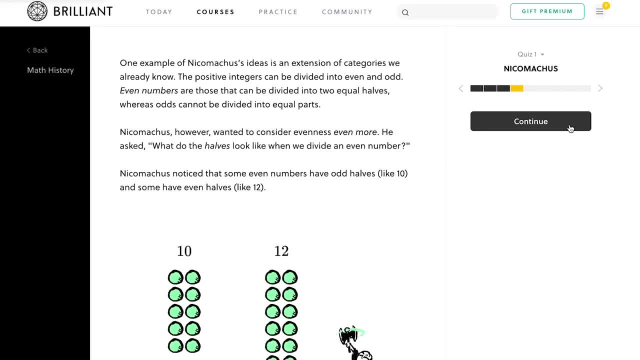 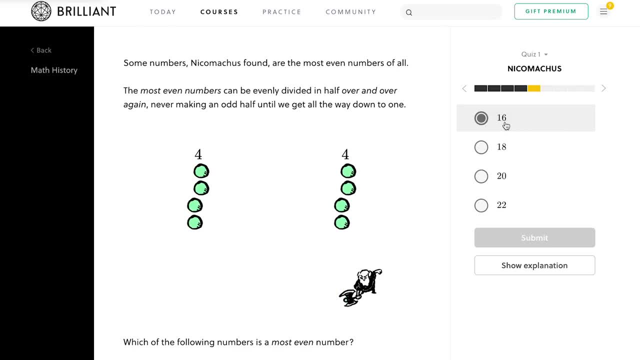 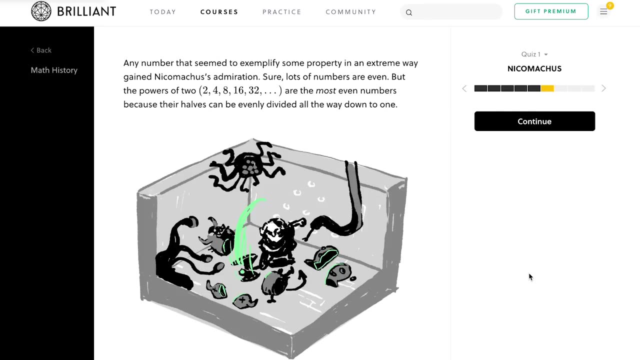 Number theory and algebra are fundamental branches of mathematics that gave rise to abstract powerhouses like abstract algebra and algebraic geometry over the last centuries. If you are interested in learning more about number theory and algebra, the fundamentals and related topics, I would recommend you to check out brilliant today. 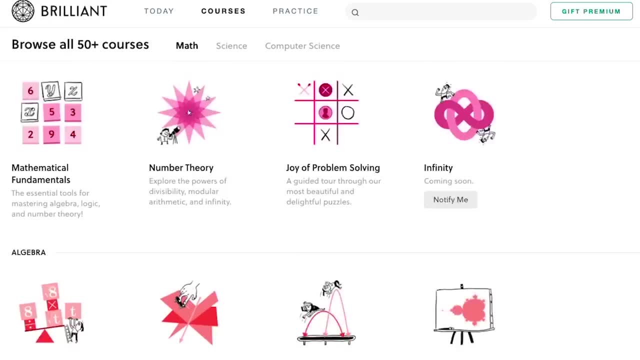 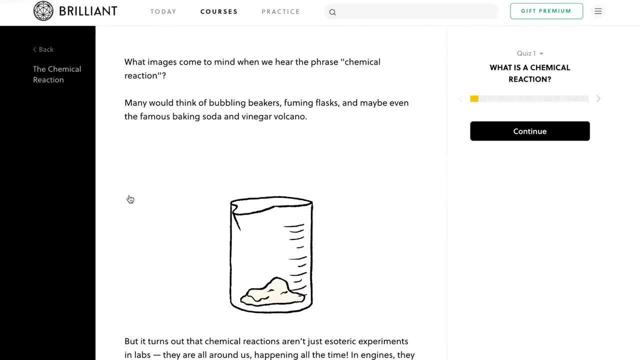 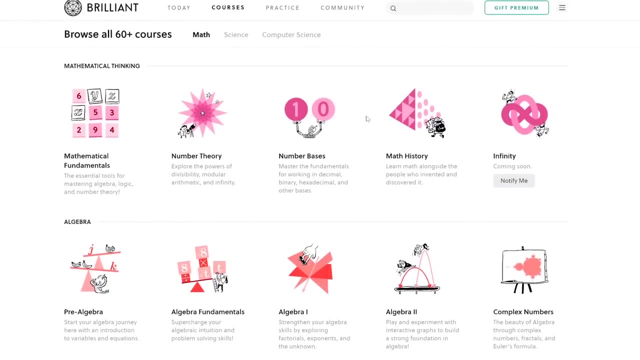 If you take a look at their huge collection of mathematics and physics problems, You might notice that this website is such a great resource for almost everything, ranging from what we did today- Special relativity- all the way to chemistry and also cryptography. right now, You would like to understand the concept of solving Diophantine equations a bit better. 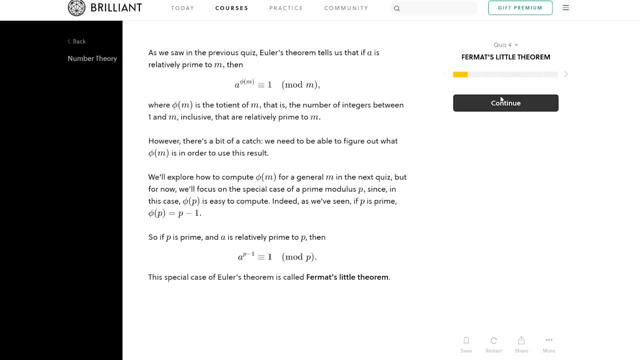 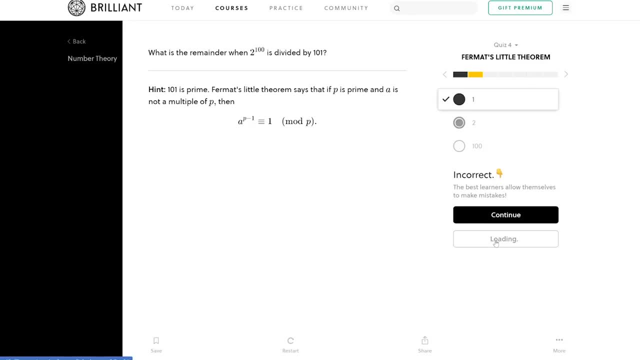 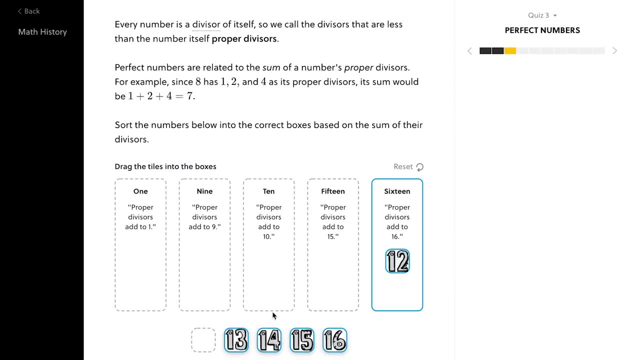 brilliant. has you covered? Simply go to their number theory based courses, put in some time and effort and check if your solution fits the provided ones. Brilliant is seriously amazing and I just love to work through their courses. Especially exciting to me is their brand new math history course, because this new format really adds a fresh twist to the exercise library. 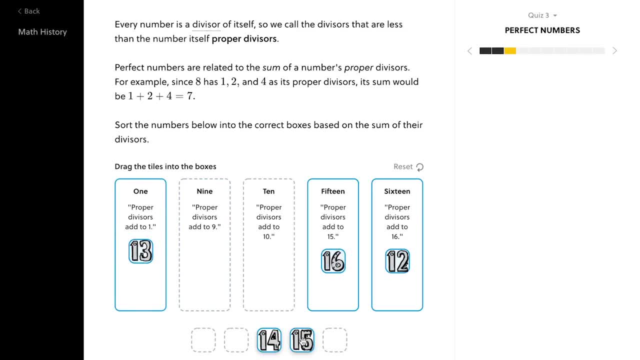 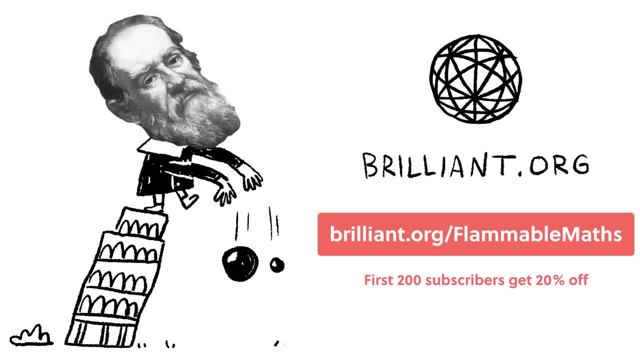 Their list of available courses grows each and every month, by the way, So I can really recommend trying out brilliant. if you are interested in trying it out for free, make sure to use the code at the top of the video's description. Best thing is the first 200 people to use the link at 20% of an annual premium subscription. 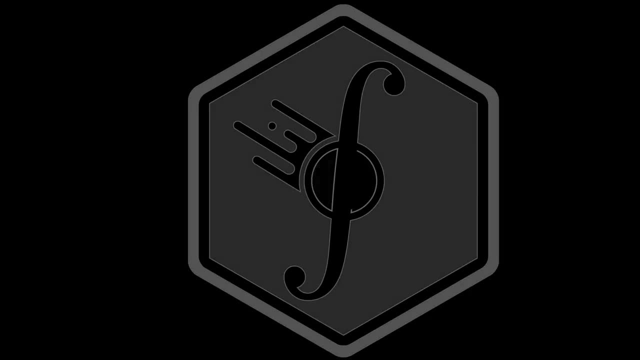 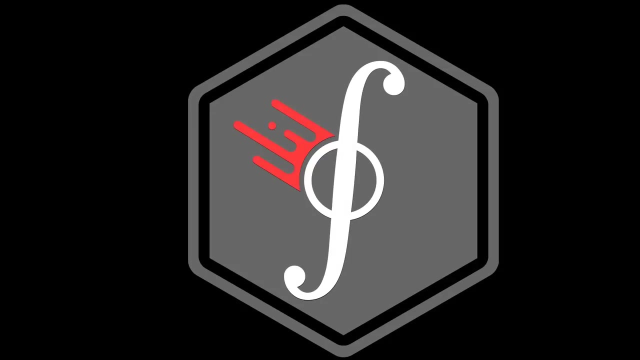 So try it out and support channel this way. if you enjoyed this video, be sure to subscribe and recommend channel Like. don't forget to check out the merch and also go over to PapaFlamme2 to take a look at the outtake video and various other.